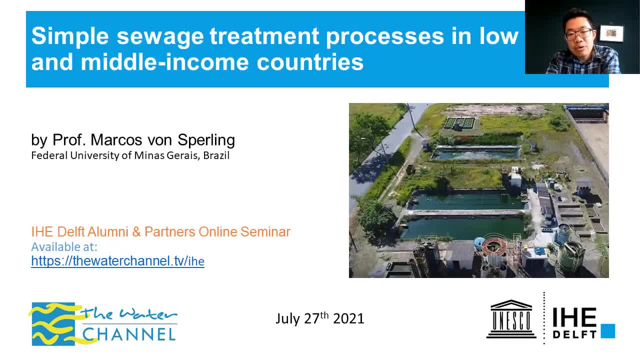 been awarded the prestigious IWA Global Water Award in 2021. And with that, our sincerest congratulations to this great achievement, dear Marcos. In today's talk, Professor von Spelling will feature simple sewage treatment processes in low- and middle-income countries In the course. 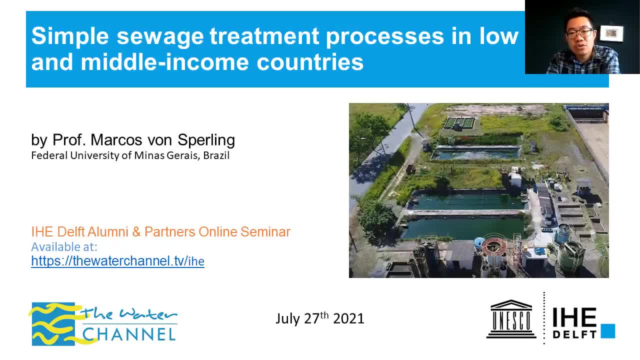 of the webinar. we look forward to hear about different low-cost solutions that are out there, what makes them suitable for low-cost and make them suitable for low- and middle-income countries, And we are also looking forward to see what the big challenges are in terms of sewage treatment needs. 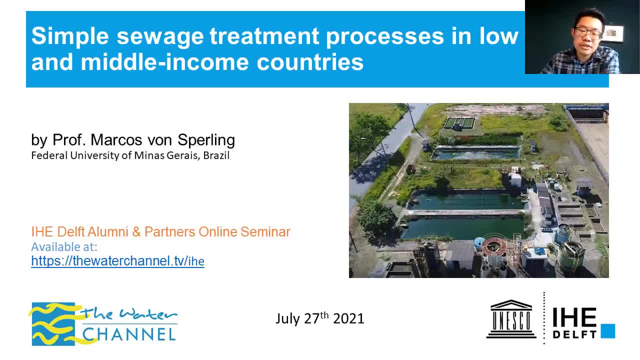 Before we begin with the presentation, I would like to take a brief moment to mention some logistics and housekeeping matters. Please could you all mute your mic throughout the presentations, And we also welcome you to have interactions with our speaker by posting questions in the chat box. 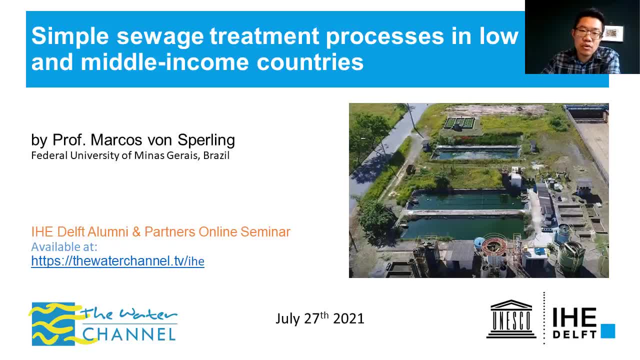 We will collect all these and address them in the Q&A session that will follow. All the presentation and recording of our webinars are available at the Water Channel website as well as the IHE dedicated website. My colleague Abraham Abishek will share the link in the chat box. 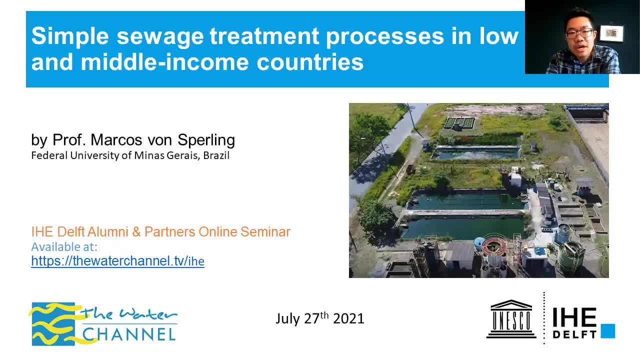 And, lastly, we would like to thank Ms Maria Laura Sorrentino, who is also with us today, for mobilizing IHE's faculty students and its very active alumni network in organizing this webinar series And, without any further ado, I would like to invite Professor von Spelling to introduce the webinar. 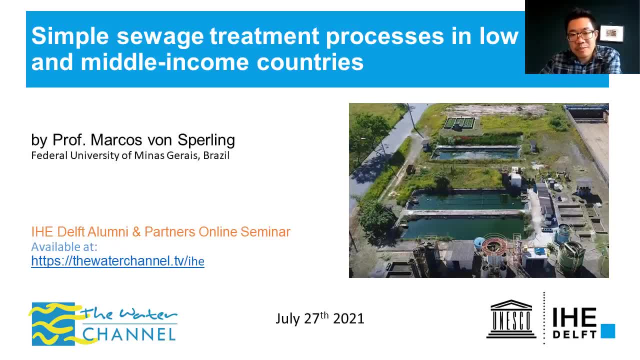 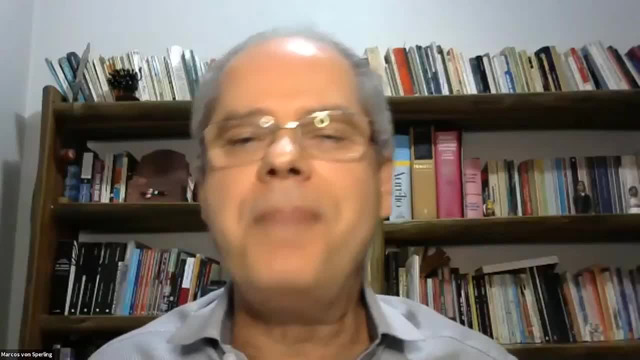 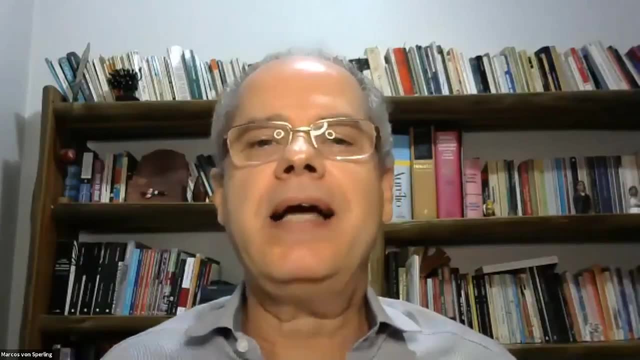 Good morning, good afternoon, good evening to so many of you. I'm very happy to be here. I see the large list of participants here. It's fantastic. It gives me a lot of enthusiasm to share a discussion with you, And thanks a lot for. 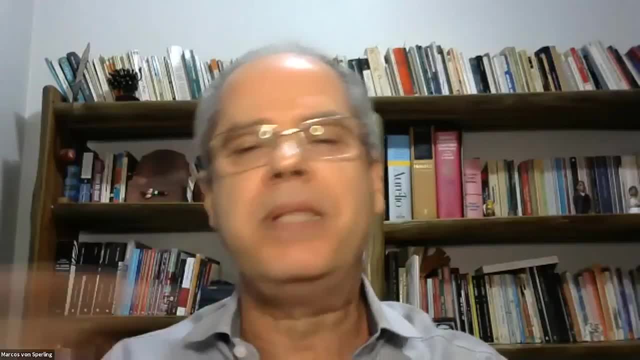 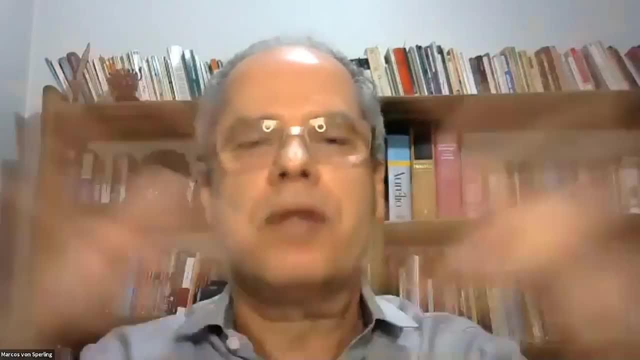 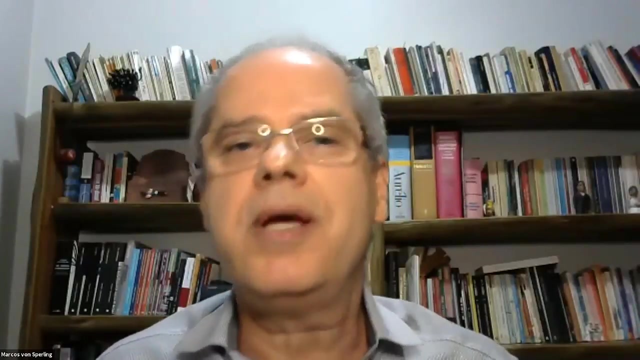 the invitation for IHE. Maria Laura, you have been superb in the connection and keeping everyone always at the same pace and joining all the large programs you have with alumnus, And also to the many friends I have at IHE, Professor Damir, who coordinated a fantastic 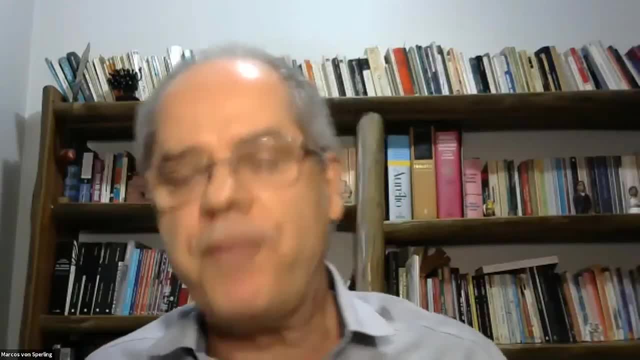 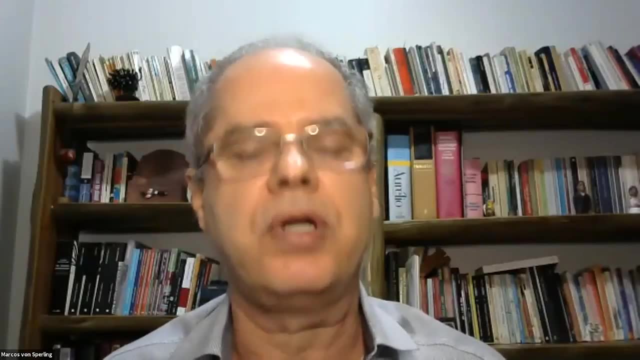 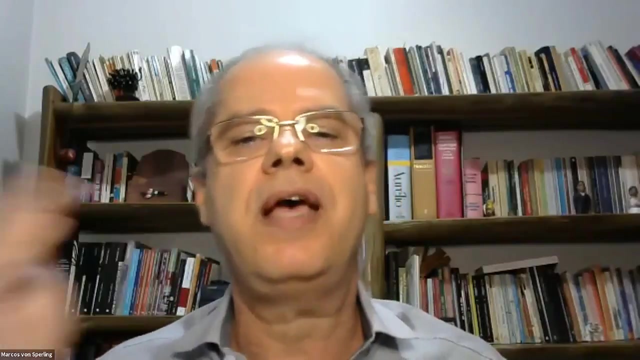 project of sanitation for the urban poor, and Professor Carlos Vazquez, who I also saw his name here. I keep contact with him because I'm a guest lecturer in a course coordinated by Carlos Vazquez and many other friends I have at IHE, other professors and the students, And at Water. 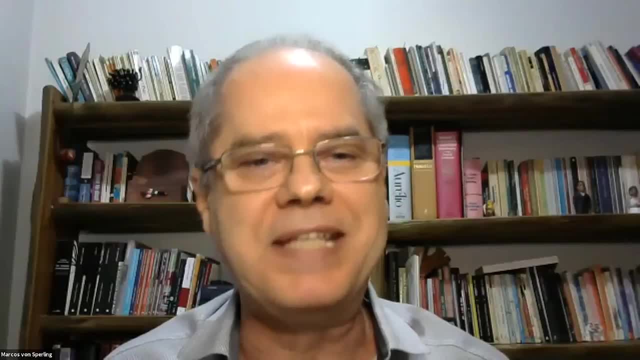 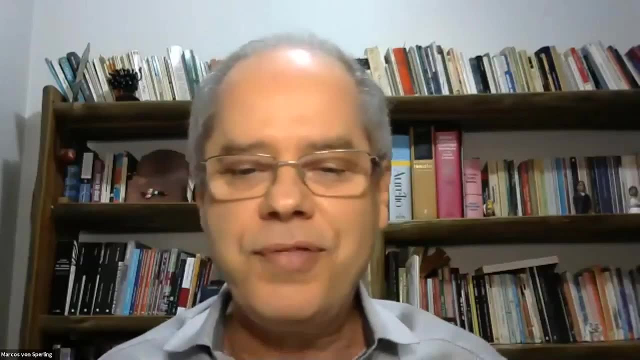 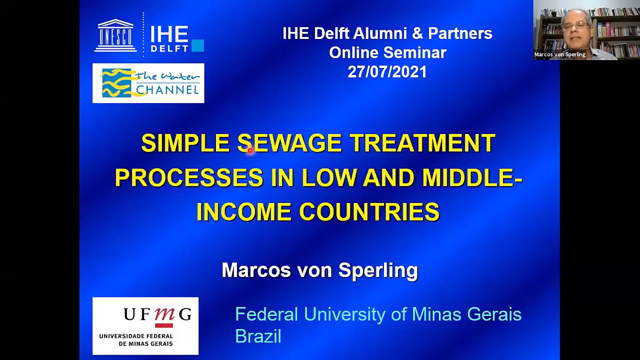 Channel. it has been a pleasure, Long and Abraham, for coordinating this, and to all participants again, So I think it gives a lot of responsibility for this talk. I will start sharing my presentation now. My presentation will cover simple sewage treatment processes in low- and middle-income. 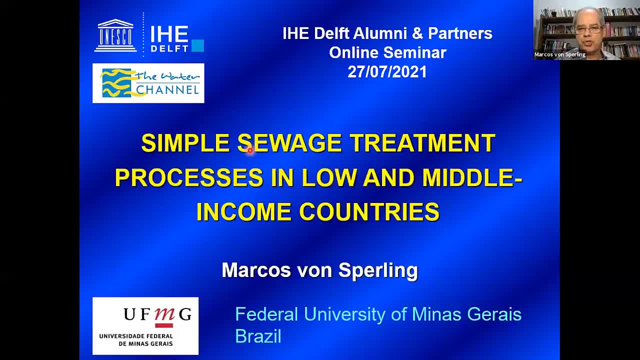 countries. So we can start sharing my presentation now. My presentation will cover simple sewage treatment processes in low- and middle-income countries. So we can see we'll talk about simple solutions. We will cover low- and middle-income countries and also. 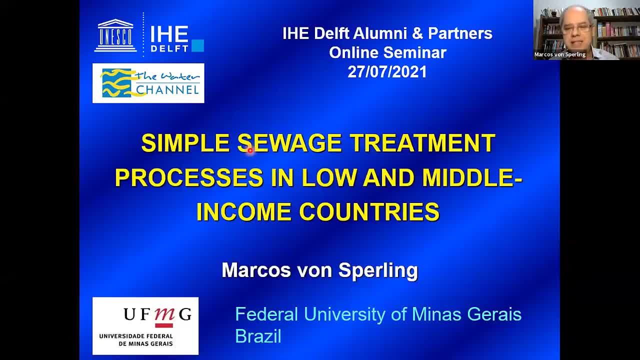 shortly I will make an association with climatic conditions, So this gives more or less the framework of what we will cover here. So, as it has been told, I'm a professor at the Federal University of Minas Gerais, Brazil. I am based in the city of Belo Horizonte, which is in Southeast Brazil. 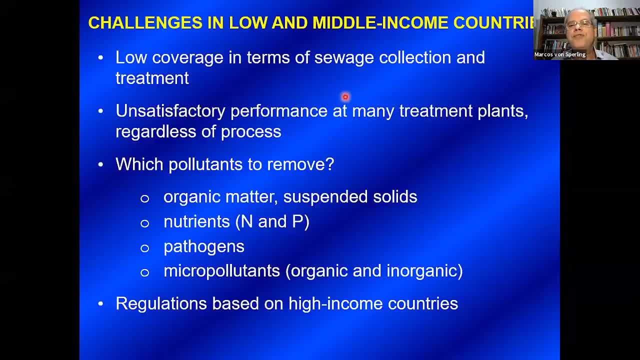 Okay, So what are the challenges we have to face in low- and middle-income countries when we're thinking about sewage treatment? Well, many, many challenges. I have just listed few of them here. In most of the cases, we have a low coverage in terms of sewage collection. 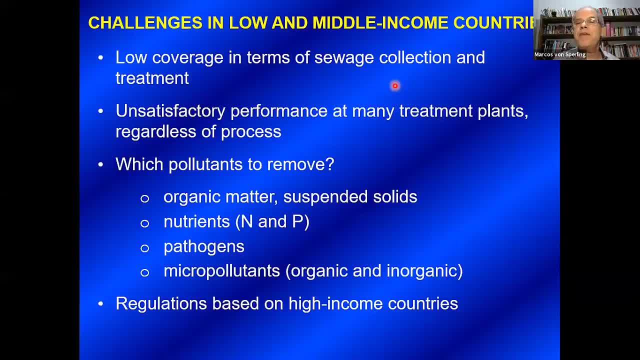 and treatment, And even when we have coverage, even when we have treatment processes, we notice that we have an unsatisfactory performance at many treatment plants, regardless of process, of activated sludge, stabilization forms and so on. In many cases we have an unsatisfactory performance. We also. we are faced with a challenge. 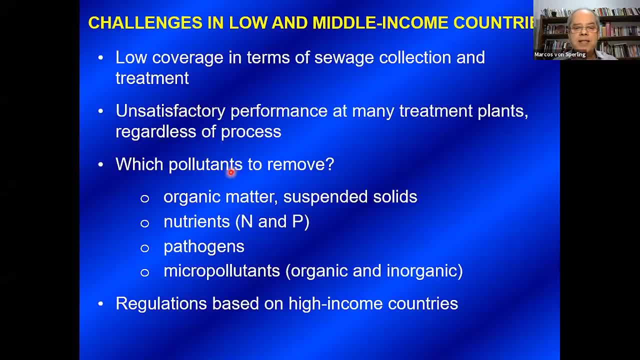 which pollutants to remove. In most of the cases we aim at removing organic matter and suspended solids. These are the major macro pollutants we aim to remove at most of our treatment plants. But we are pressed on many sides, especially from the more developed countries in which they are. 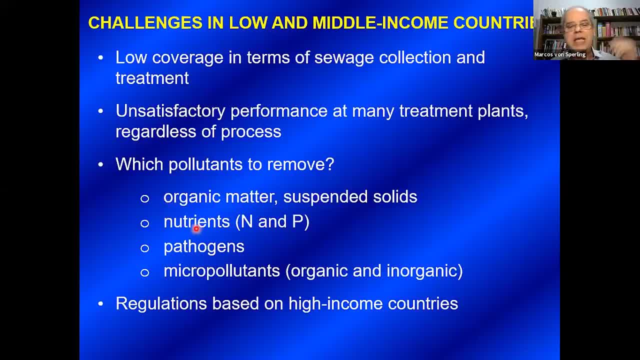 almost on a routine basis now removing- or for many years removing nutrients, nitrogen and phosphorus, thinking in terms of eutrophication control and other aspects related to nitrogen and phosphorus. We also have the challenge of removing pathogens In many cases. 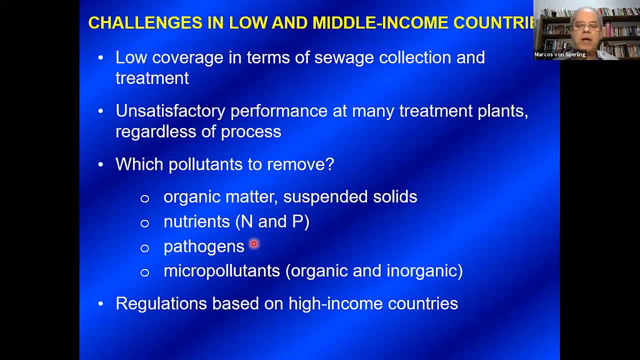 they are very important, especially in our condition of less developed countries or middle-income countries, And micro pollutants- we observe, we read the literature now is focusing on removing micro pollutants, that developed countries are talking about micro pollutants. How can we organize such a huge agenda and put this into perspective and select what shall I do? 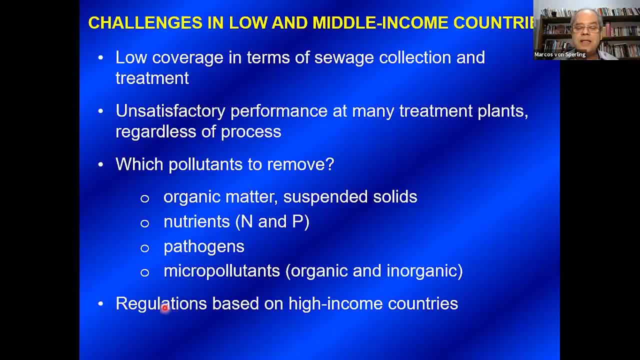 next, Okay. and also, we see that in many cases, the regulations are based on high income countries, So many countries of middle and low income countries. they simply copied legislations from high income countries, which, as you can see, makes things very difficult. if we have to remove all of this, Okay. 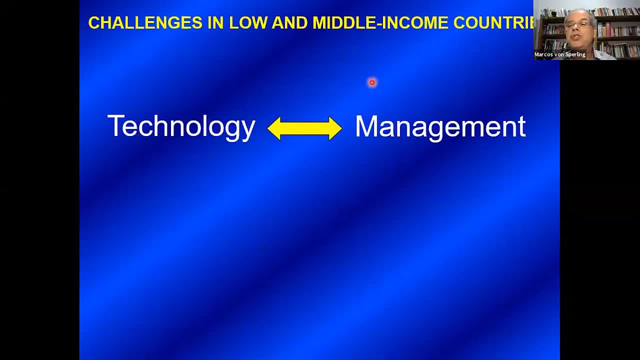 And again we could be talking about technology and management. I will talk mostly about technology now, But I should take the risk of saying that most of our problems are related to management, Because technology, as we will discuss, we have a large array of possibilities. 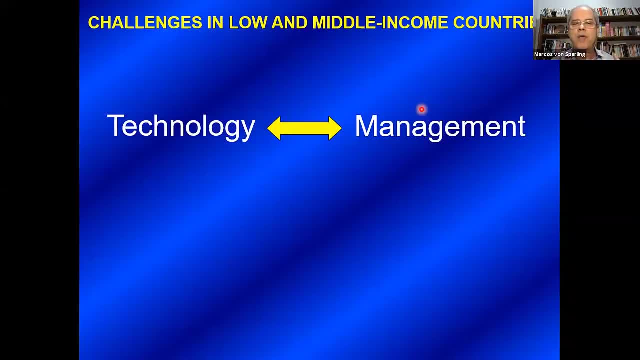 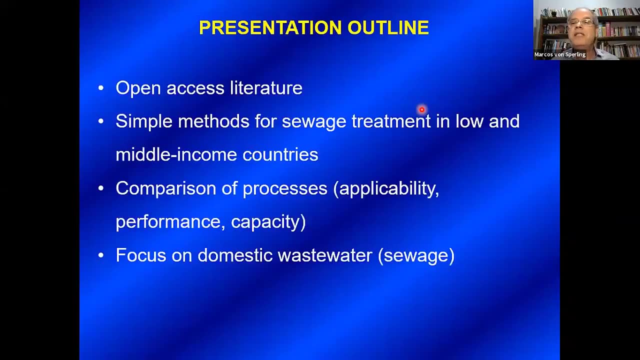 that we can use. So choices are not our problem. Okay, So management problems are in most of the cases what we have to face. the presentation outline I'll have, so I will shotly show in open access literature, And Long has already mentioned about some publications, some books, I 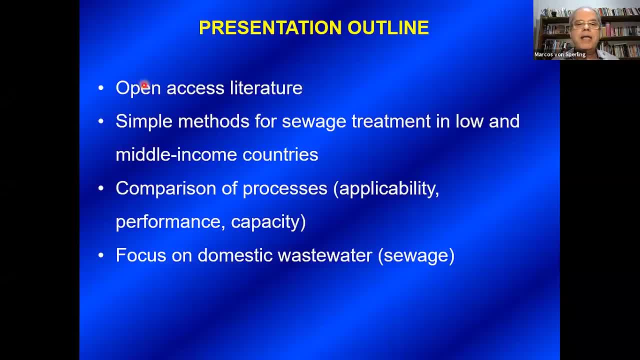 I have been involved with. I will share with you the links for these open access literature. We'll cover it as I told. simple methods for sewage treatment in low and middle income countries. Of course, we will not have the time to describe the treatment process. 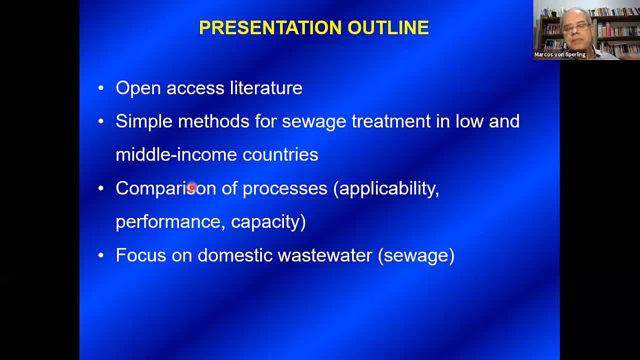 So most of the time it will be, I'll dedicate to discuss about their applicability, a comparison in terms of performance and capacity of removing pollutants, And the focus will be mainly on domestic wastewater sewage, So we will not cover, for instance, industrial wastewater. 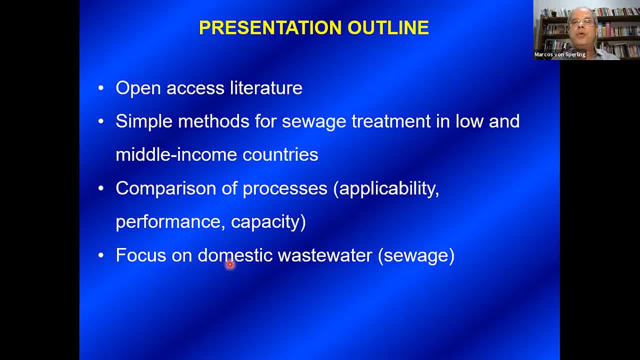 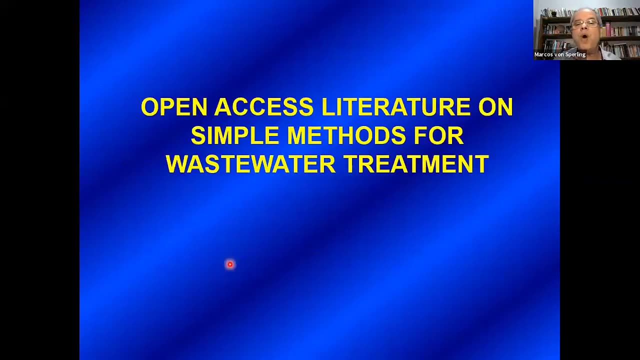 And also we will talk about more on a communal solutions or municipal wastewater, urban wastewater. We will not be able to cover onsite treatment just for one household. okay, So it will always be for a group of households. So what are? we could say, open access literature. 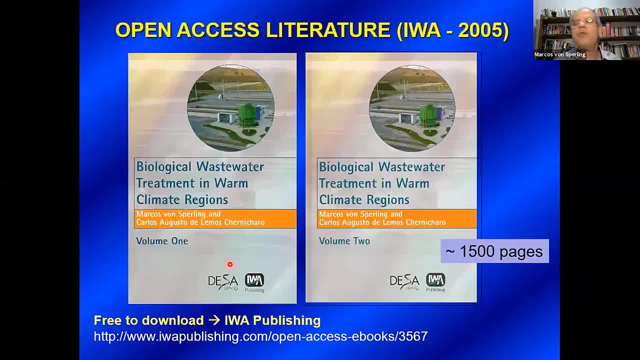 on simple methods for wastewater treatment. Okay, there are many books: IET, DELF, Damir Carlos Lopez. they have made fantastic books, Some of them available as open access. I'm listing here a complimentary possibility published by IWA, International Water Association publishing. 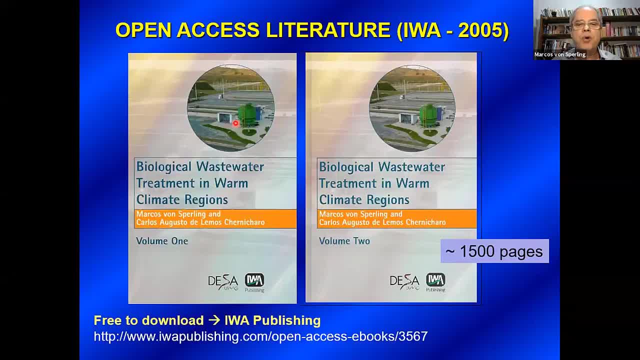 So we start IWA. We started in 2005 with these books here, which are called Biological Wastewater Treatment in Warm Climate Regions, Volumes 1 and 2.. They are large books. Summing up, they have more or less 1,500 pages. 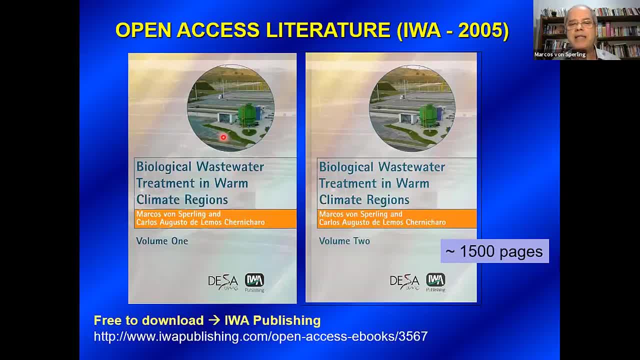 In 2013,. we negotiated with IWA in terms of asking them to make them freely available to everyone everywhere in the world. So they are now, or for some years from now, they are open access. You can see the links: the link here: 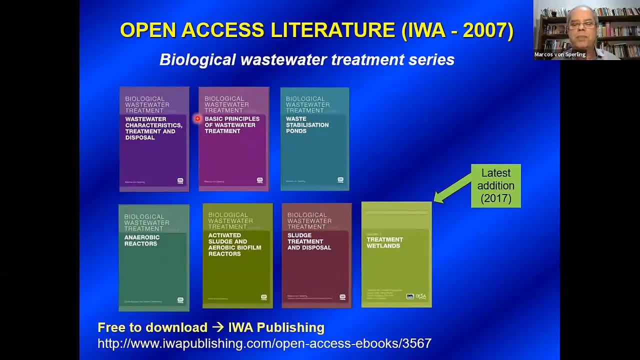 Some years after we launched the large books, the two volume books, IWA Publishing decided to split into a collection which they called Biological Wastewater Treatment Series. So you can also download Volumes 1 to 6.. So these are the treatment processes we covered in the series of books. 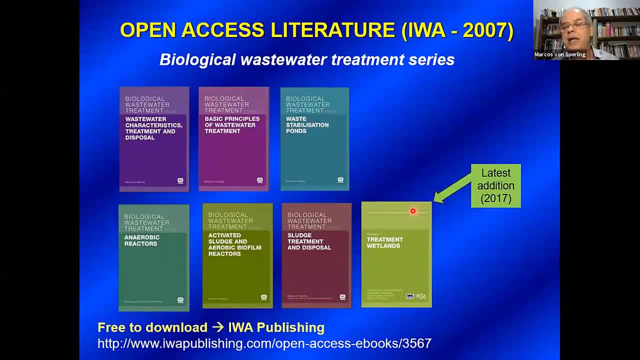 And, very interestingly, later on in 2017, a group of people from IWA, from the wetlands specialist group. they made a task force and they made Volume 7 for treatment wetlands, which was the latest addition and very welcome. 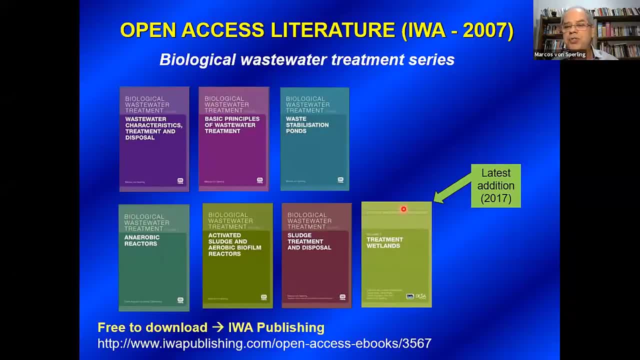 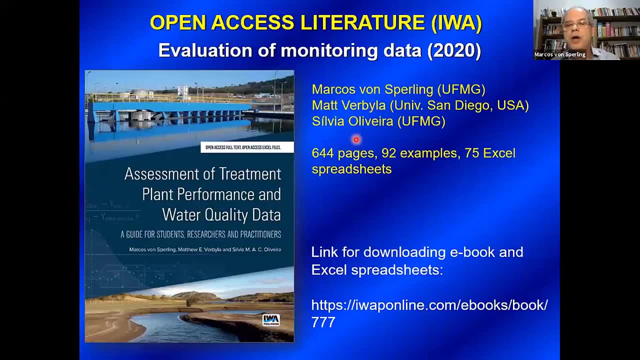 And we have for these treatment wetlands a Spanish version and a Hindi version as well. And lastly, Last year I published with other colleagues- one from the United States, another one from the same university- this book Assessment of Treatment Plant Performance and Water Quality Data. 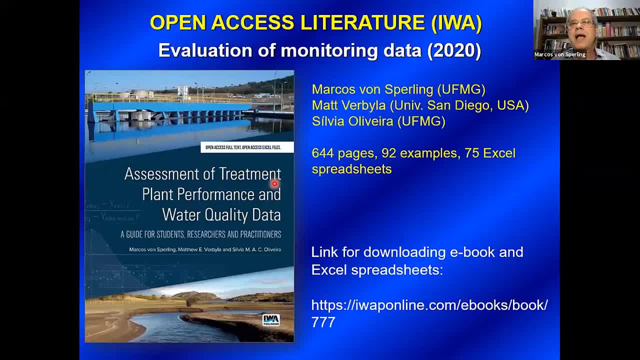 So this is mainly for helping people to plan monitoring works, how to interpret monitoring data, how to use, how to connect statistical analysis with evaluation of a performance Of a treatment plant, and also quality of rivers, water quality in rivers, lakes and so on. 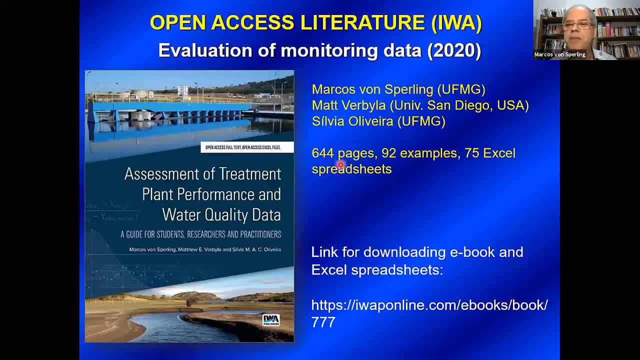 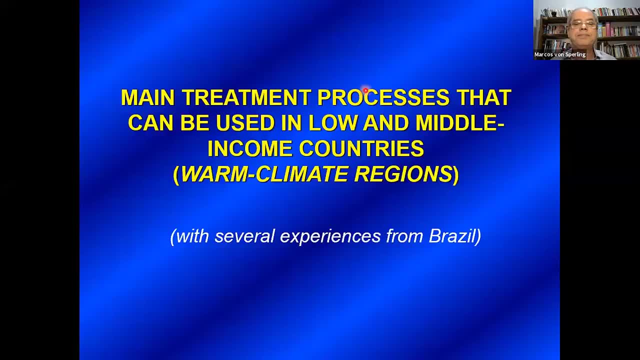 So this is also somewhat large book- 600 pages- and many excel spreadsheets freely available for downloading. Okay, So now we're coming to the processes. I would like to cover Only the main treatment processes. We have a very large list of possibilities. 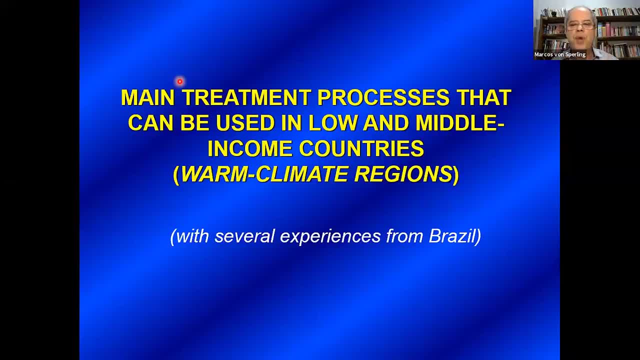 We will cover only the main treatment processes, Only the main treatment processes. We have a very large list of possibilities. We will cover only the main treatment processes. We will cover only the main treatment processes, most used ones, And I come from a warm climate region. Many of you come from warm climate regions. 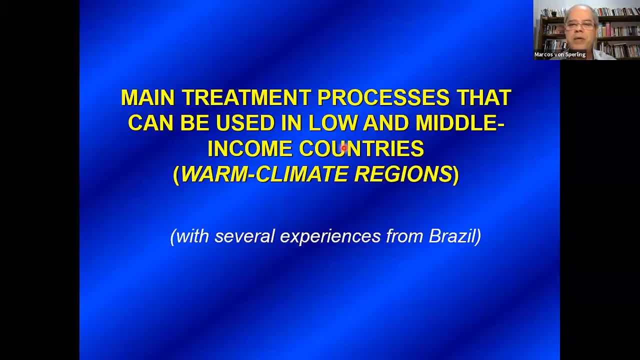 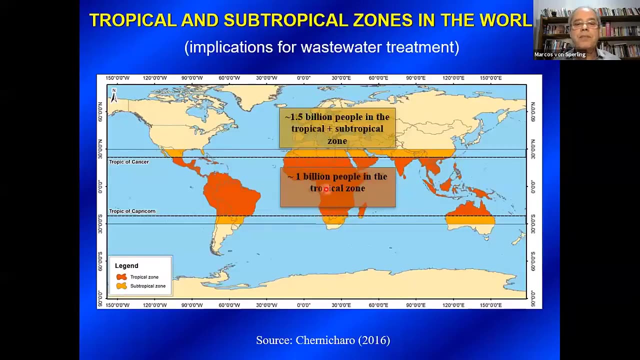 as well. So I will make an interaction between low and middle income countries and the climatic conditions. I come from Brazil. I will quote several experiences from Brazil, many those in which I have been involved with Okay. So if we think in terms of climatic conditions, 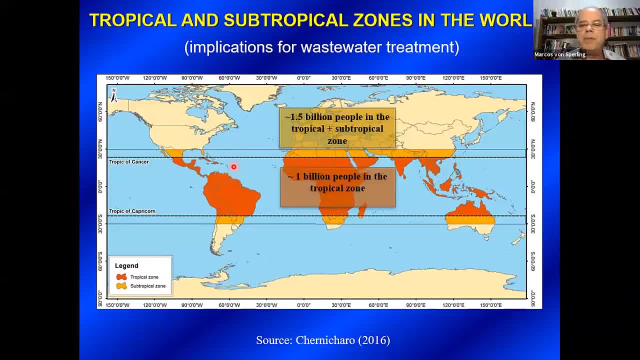 1 billion people in the world. more or less 1 billion people live in the tropical zone, You know. if we also include subtropical zones, this adds up to 1.5 billion people. So, of course, if we think in terms of biological wastewater treatment, this makes a difference. 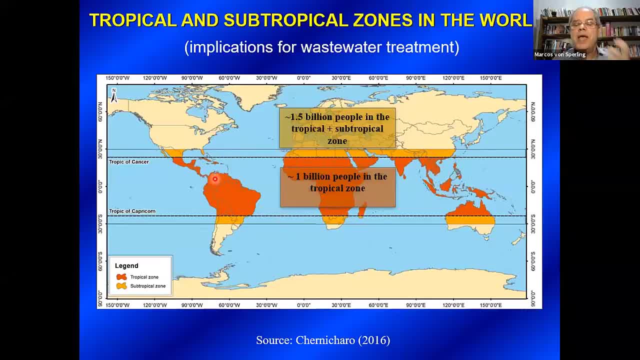 And what are the possibilities we can use if we have very favorable climatic conditions, meaning high temperature and in some cases also high sunlight penetration- and the need for simple solutions. So we are going to discuss about that. So these are the statistics from Brazil. We still 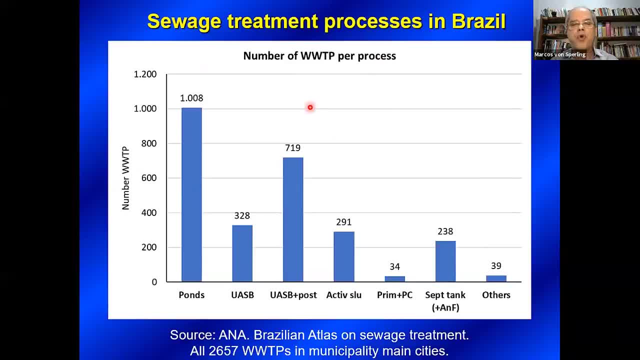 have a lot to do in terms of wastewater treatment coverage, But this is just to highlight to you- this is one of the several slides I have about this. I'll just show this one- The number of wastewater treatment plants per grouping of treatment processes. So stabilization points. 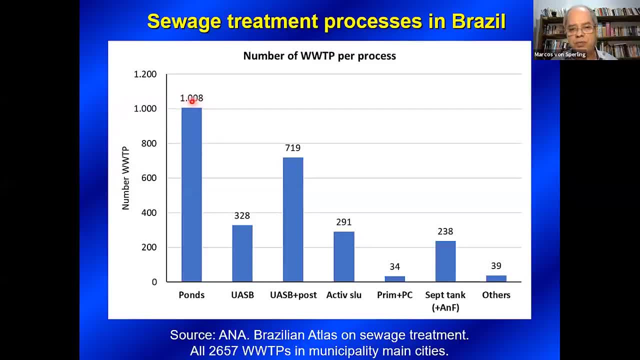 are the most widely used treatment process in Brazil. We will discuss about them. So in the sequence upflow, anaerobic sludge, blanket reactors, UASB reactors- and in the sequence we will talk about the most widely used treatment process in Brazil. 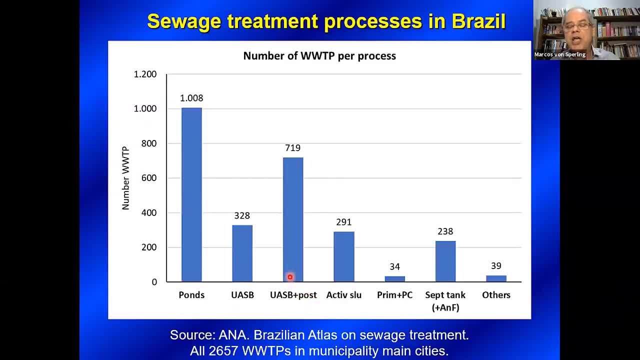 So the first one is the anaerobic treatment process. So the anaerobic treatment process is either alone or in most of the cases, and preferably followed by a post-treatment stage in order to improve the effluent quality. If we sum up these two, you will see that anaerobic treatment 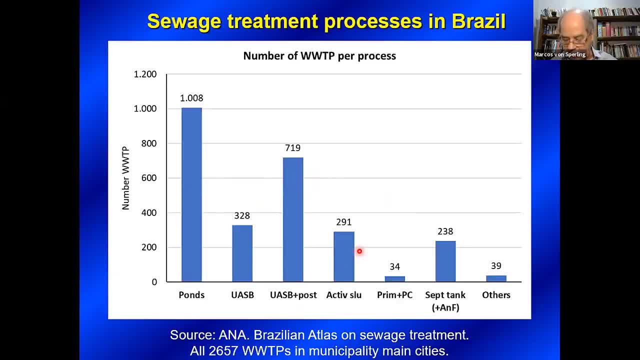 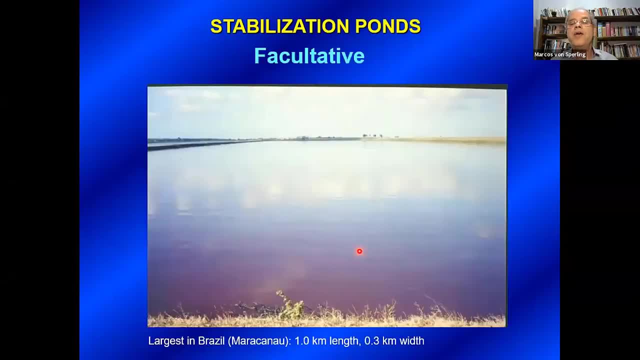 is widely employed in Brazil thanks to our favorable climatic conditions. And then we have stabilization points, Okay, Facultative points. They are the most widely used variant, not only in Brazil, but they are hugely used in many, many countries, If we think in terms of United States. 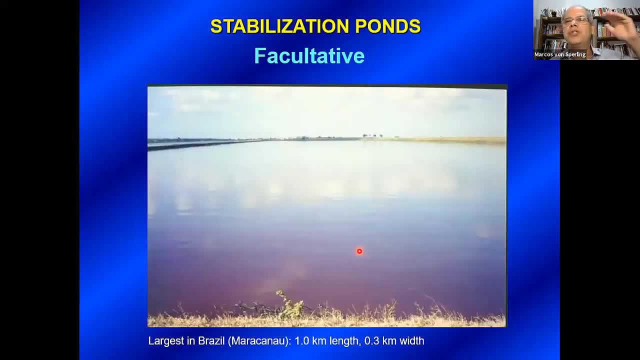 we should think. well, they don't have good climatic conditions in the north of the United States. There is a fantastic map- I won't show here because of time- showing 8,000 stabilization points spread all around the United States, from east to west, from south to north. So regardless. 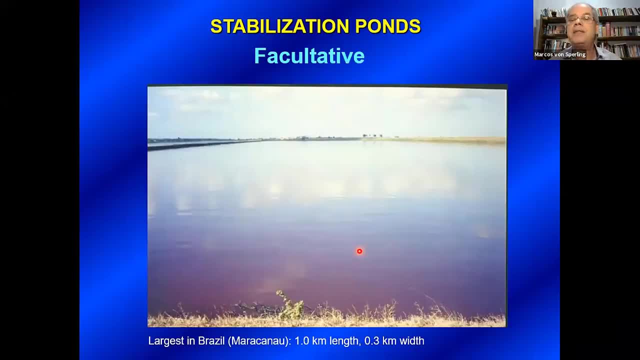 of climatic conditions. they are there, They are being used, But, and also, for instance, in Australia, they are the dominant treatment process. In France, more than 3,000 stabilization points. Okay, But of course they have their difficulty, as we will discuss. They are very. 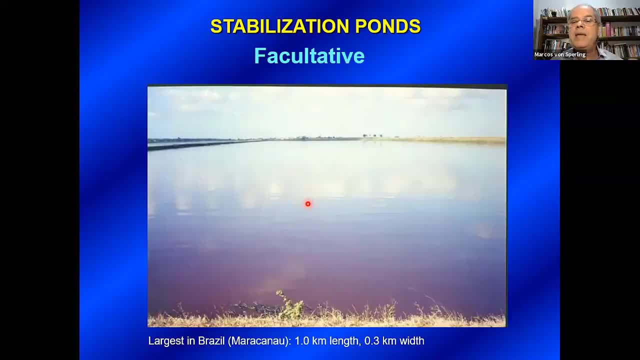 simple treatment process. They are limited in their capacity of removing organic matter, So we don't find very large treatment efficiencies, but they are able to remove many pathogenic organisms, So very important in terms of this. The major problem is the large land requirements. 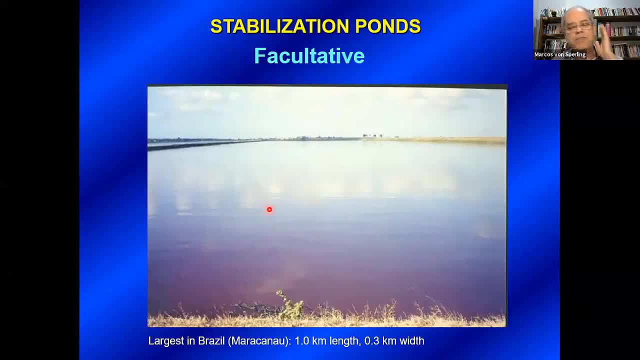 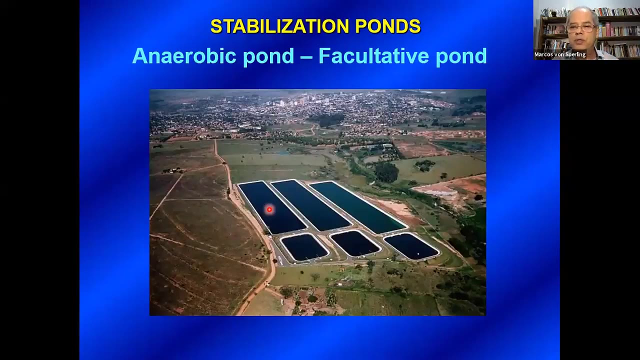 as we will discuss. So facultative points, very important in many countries which are affected here by all the participants who are joining this presentation. Okay, Because facultative points alone, we could call them primary facultative points. They take up a large area. One possibility to decrease the total land requirements would be to start. 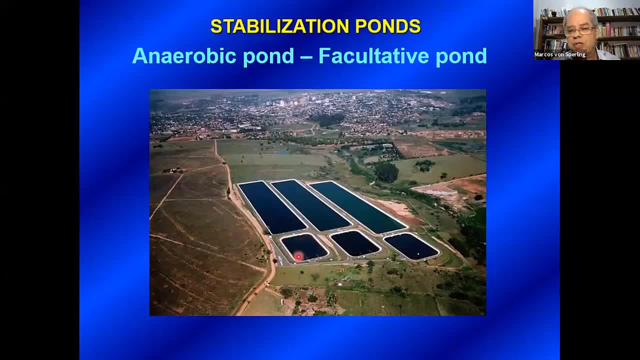 the treatment using anaerobic points. So anaerobic points could be a possibility, And then you could remove 50, 60%, sometimes even more, of the organic matter in the first stage, of anaerobic points And then decreasing the land requirements for the facultative points. So that's. 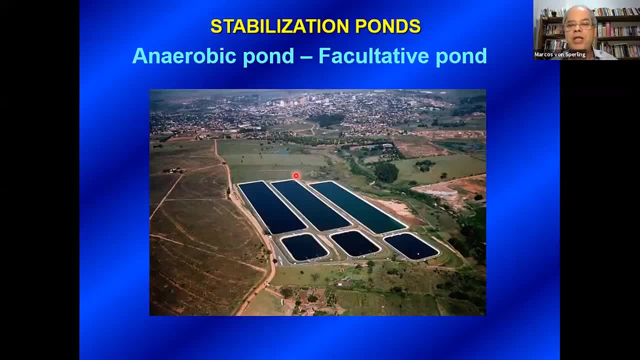 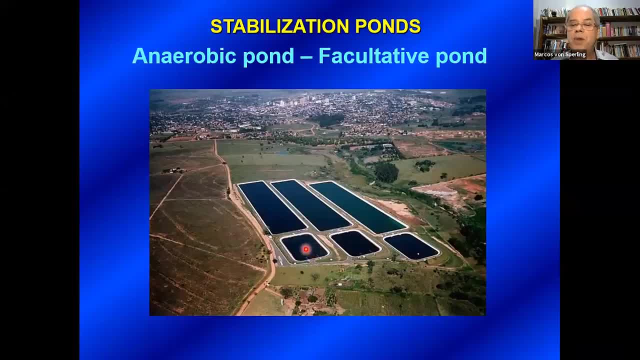 We have anaerobic reactors. We have anaerobic reactors, We have anaerobic reactors, We have open reactors And we are concerned about problems with bad smell. So you can see here that ideally, these treatment processes should not be surrounded by population. 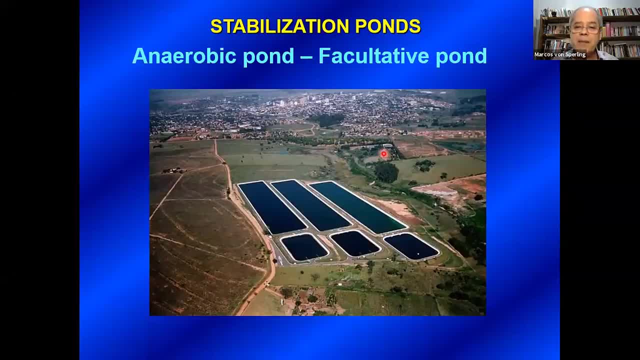 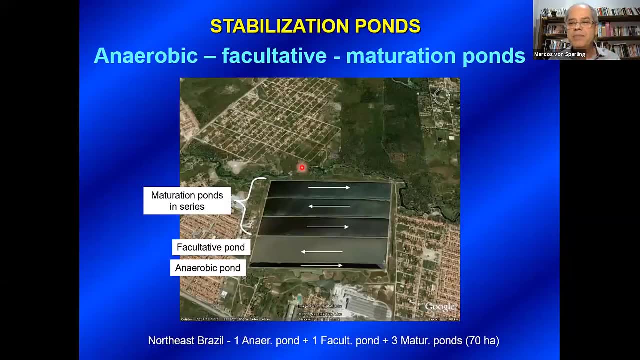 because there could be complaints related to malorders. Okay, Now we improve our capacity. If we aim to remove pathogenic organisms, we can include the stage of maturation points. This is the largest system we have here in Brazil. It occupies 70 hectares- 70 hectares. 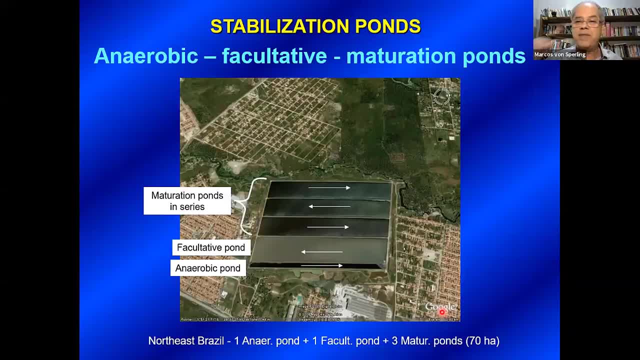 There are much larger points. in Argentina They have 300 hectares, In Australia 300, 400 hectares, But in our case that's the largest system. Notice that if we are aiming to remove only organic matter, just the anaerobic point and the facultative point could be sufficient. 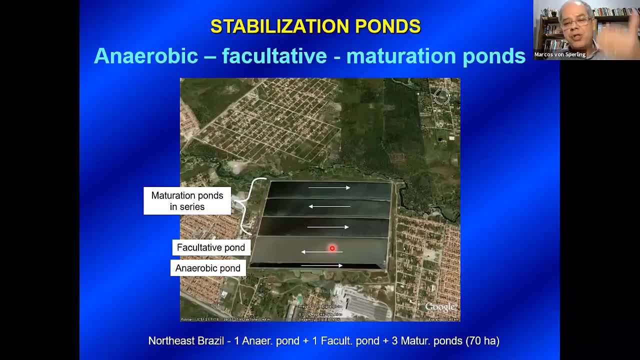 If we want to add an additional objective, which is removing pathogenic organisms, and then mainly removing all categories of pathogenic organisms- pathogenic bacteria, viruses, protozoan cysts and helminth eggs- maturation points will do a superb job, Ideally. 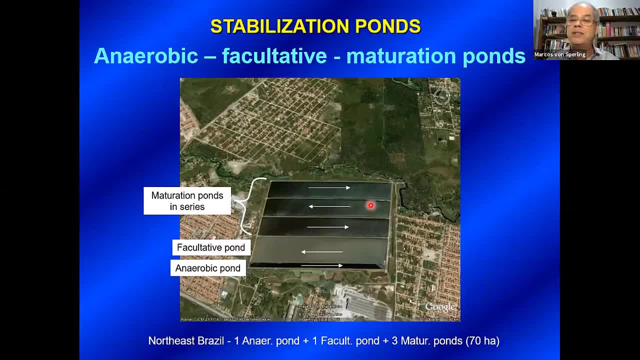 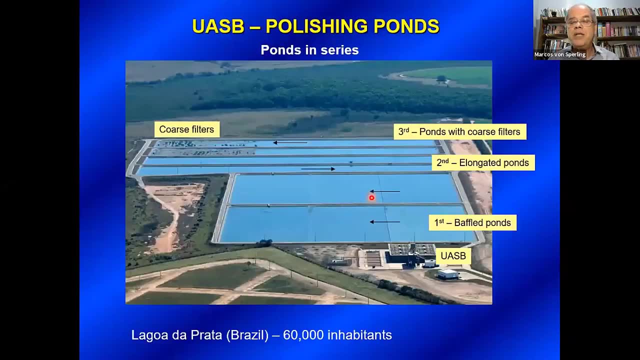 they should be arranged in series And, as you can see, it takes area. There are extensive treatment processes, natural treatment processes In Brazil. since I told you that we are applying upflow anaerobic sludge blanket reactors, UASB reactors, one possibility could be to have the 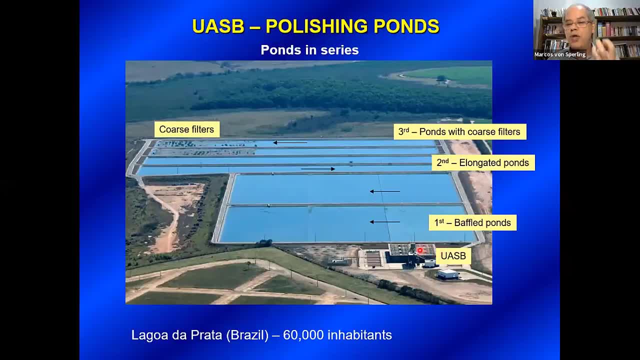 first stage, Instead of having anaerobic points, we could have a closed reactor, controlled reactor with higher removal efficiencies compared with anaerobic points, And then we could have the post-treatment, either to improve in terms of organic matter removal and, most importantly, 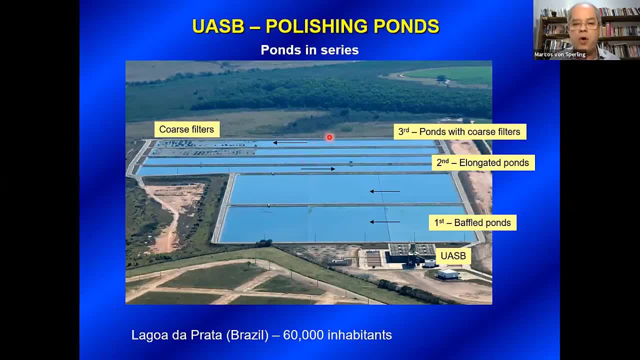 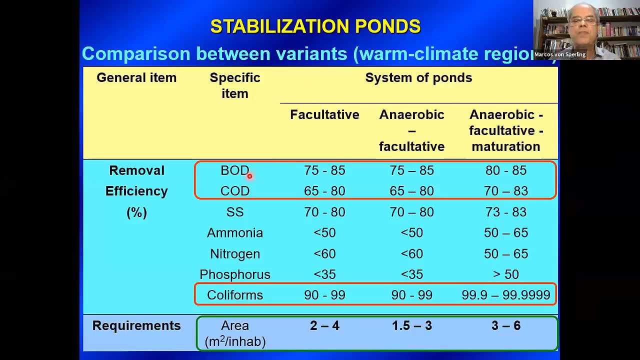 also incorporating removal of pathogenic organisms. Okay, So this is a summary of important elements in the decision process. Which process should I use? So these are typical removal efficiencies of the main arrangements I showed to you in terms of BOD, COD, in terms of coliforms. 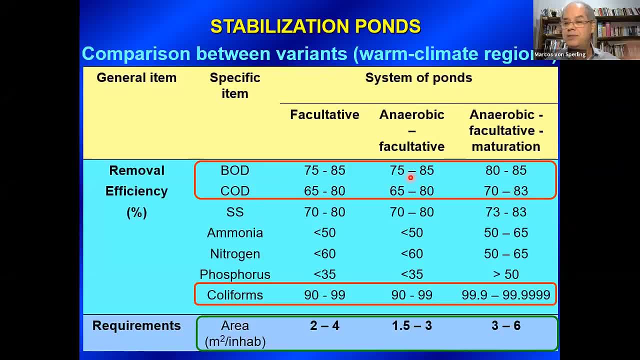 So you can see well, the removal efficiencies are not spectacular. They are in the range of 75% to 85% for BOD, slightly less for COD. We are not able to remove well suspended solids and also nutrients in these typical arrangements, But we are able to remove very well coliforms. 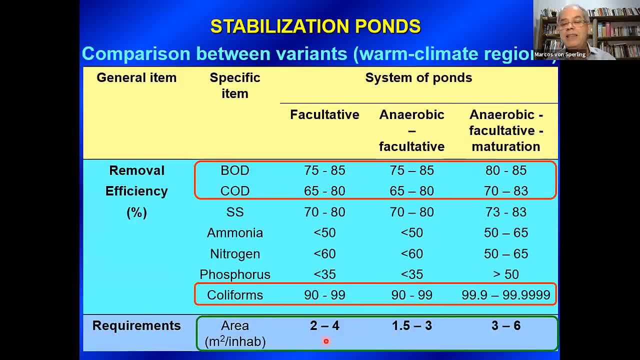 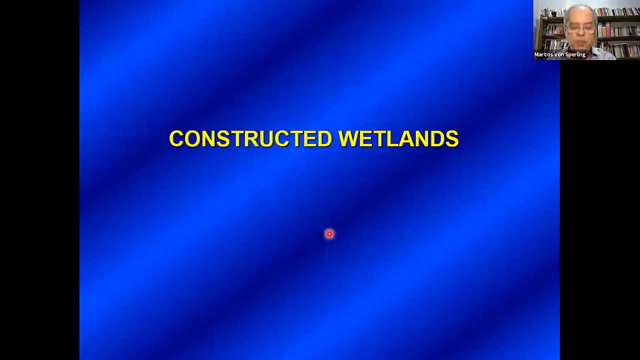 especially if we incorporate maturation points And the land requirements in warm climate countries are between two to four square meters per inhabitant if you apply only facultative bond and more if you incorporate maturation points, Constructed wetlands, a treatment process that 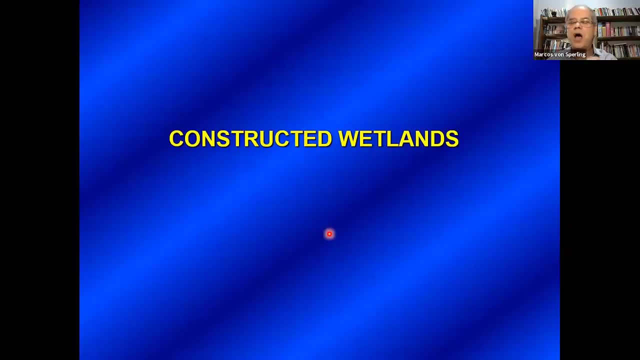 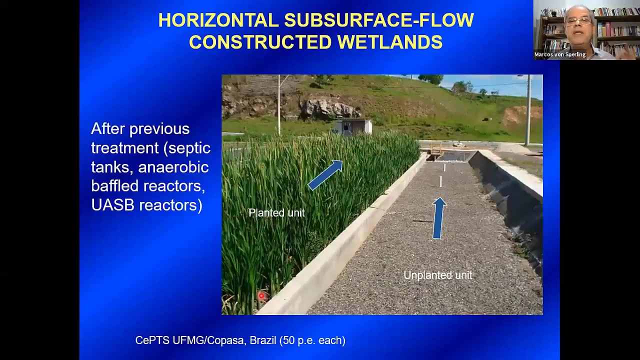 is increasing the number. We have thousands, of, tens of thousands of units such as that in operating in Europe, in North America and in other continents as well. A widely adopted treatment process are the horizontal subsurface flow wetlands. They need to come after a pre-treatment stage. 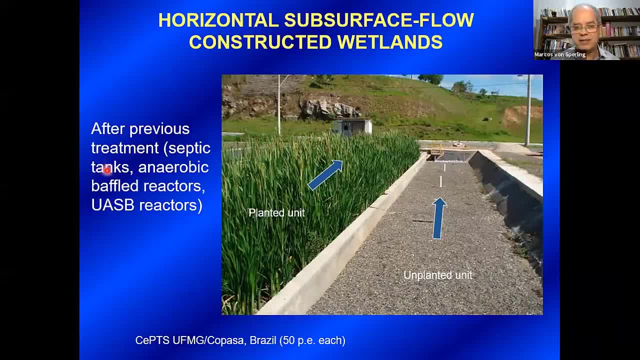 In most of the cases after septic tanks, But they are also applied after anaerobic baffled reactors And in Brazil we are starting to apply them after UASB reactor as an additional possibility. They are a natural process. They are a natural process. 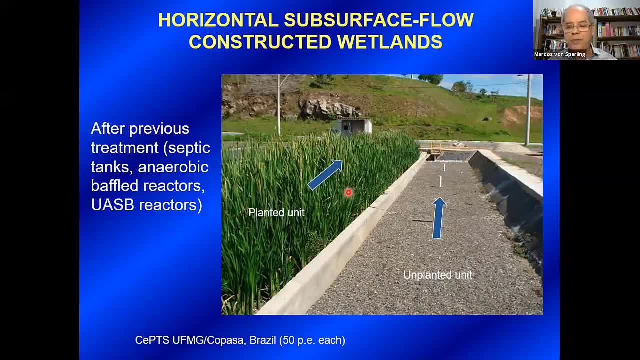 They will use a lot of area as well. Here I'm showing one in our experimental site. This one is for treating 50 inhabitants, 50 population equivalents. That's the real wetland, because it has plants. That's just a controlled unit for purpose, for research purpose. It's an unplugged unit. 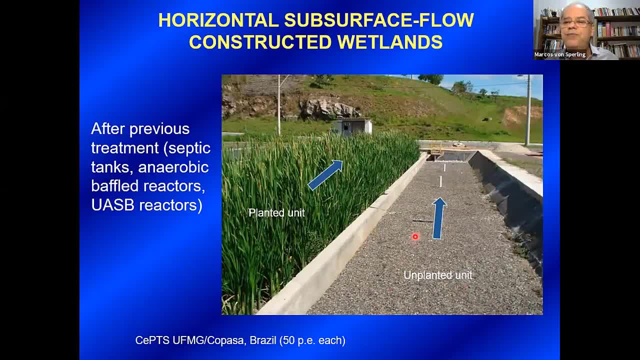 it is a filter And then the liquid falls this way as subsurface flow. So this means that you don't have wastewater and it returns to the soil and it is a practice field flowing on the surface. that's a positive thing. we can discuss about clogging later on. that's a 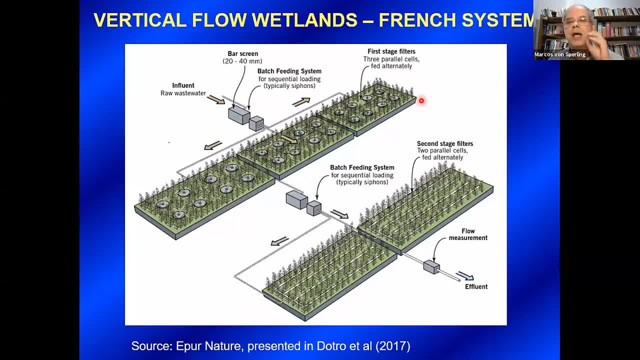 system i like very much. i think it has a superb possibilities for application in our climatic conditions. it's the vertical wetlands, but the french system of vertical wetlands- so that's how they are called in the international literature- the french system of vertical wetlands. so the wastewater is discharged on top of the surface. we have a first stage here. 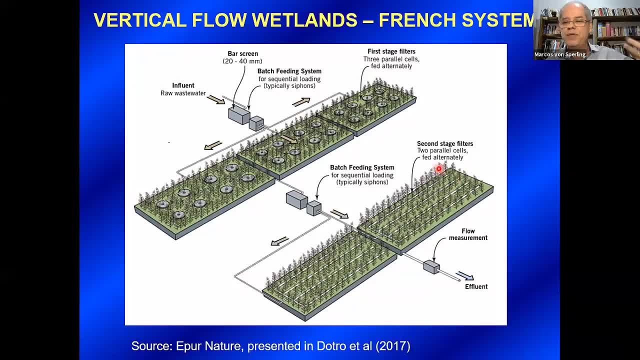 a second stage here for improving the effluent quality. you can see that in the first stage we have three units in parallel and they work on an alternated basis. this filter is working on an alternated basis and they work on an alternated basis and they work on an. 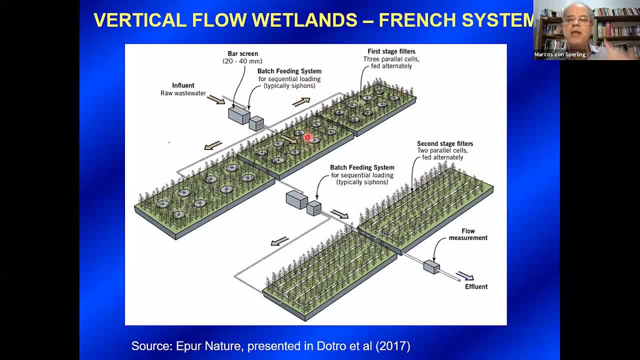 and the two others are resting, and then we start operating. after some days we start operating this one and this starts to rest, and so on, and the filter in operation is fed on an intermittent basis on a batch mode. this brings important characteristics we can discuss later on. 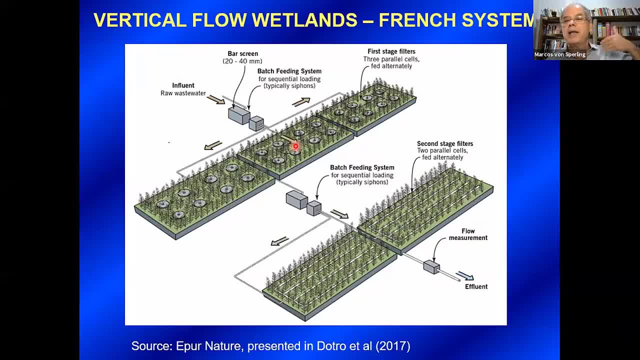 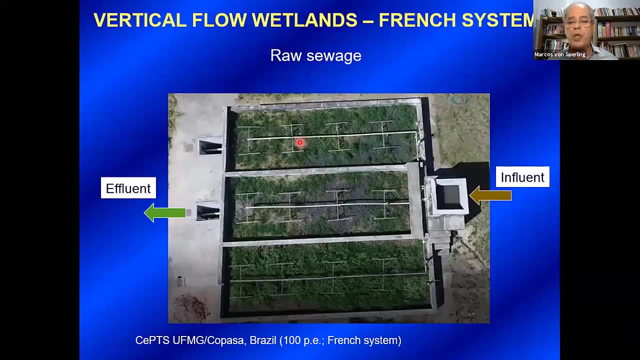 but in this type of system also, we can remove well organic matter, but we can also nitrify, remove ammonia nitrogen, which is an important thing. this is from our uh research center as well. an example we adopted only the first stage here is for 100 population equivalents. 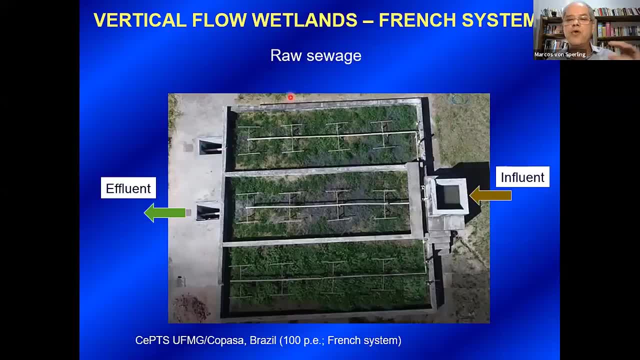 you can see a top view of the three units comprising the french system of vertical wetlands and we, and also the french in their former colonies, in their current territories, they're doing research on. do we really need, uh, the second stage? we think no, if we have good climatic. 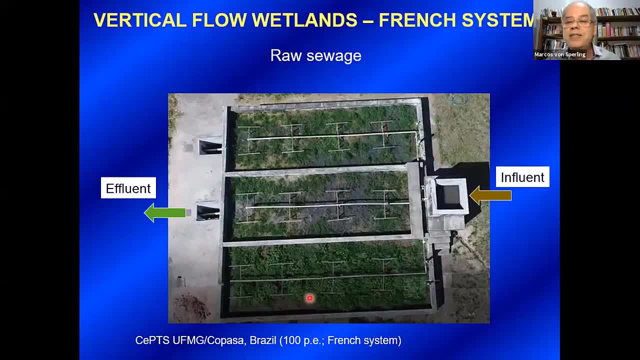 conditions. and now the further question is: do we need three units in parallel? can we just use two units because of the favorable climatic conditions? usually this takes up one square meter per inhabitant. just the first stage, but if we adopt only two filters, you come down to: 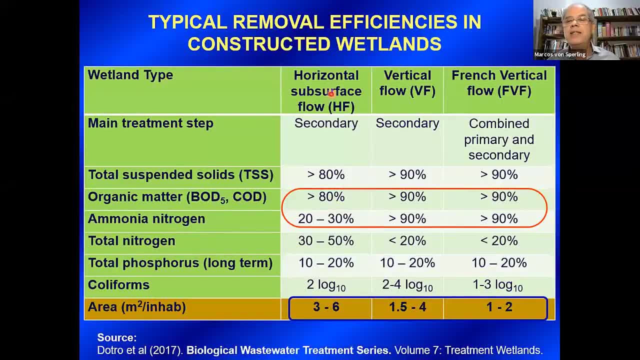 0.7 square meters per inhabitant. so again, this is a summary. we won't have much time to discuss uh tables. you can see that the removal efficiency in terms of organic matter, just of the uh wetlands stage, is very good. i forgot to emphasize when i talked about the french vertical flow wetlands. 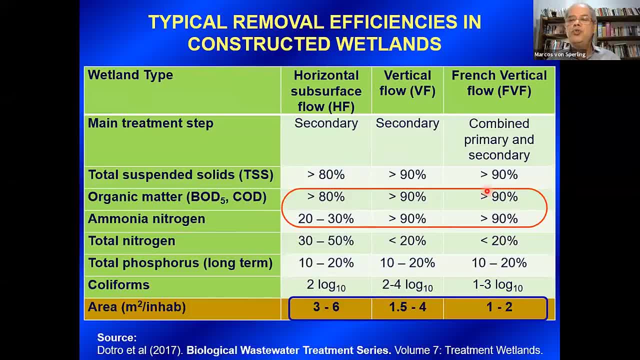 is that they treat raw wastewater. you don't need anything before, you don't need septic tank feed, they don't need to use man-made systems and we also can verify that the flow is very efficient. and if there's a lot of areas where there is a lot of contact fixing going on in the 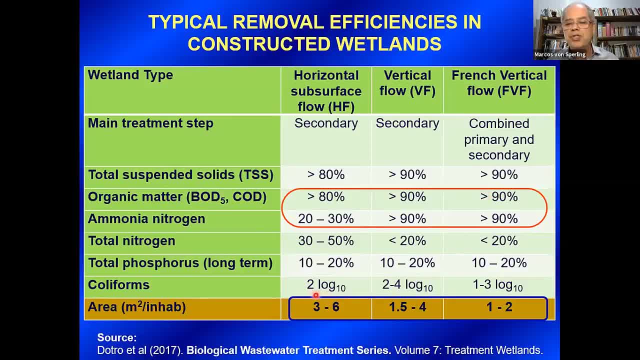 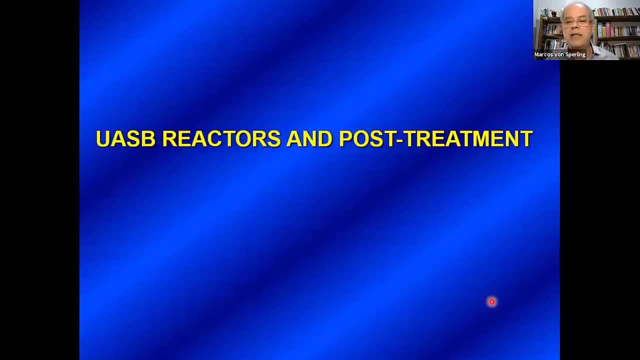 water, they're not going to be affected. so this is to make sure that- and this is the reason why, um we adopted uasb reactors- buffled anaerobic reactor. they just receive raw sewage and this is very, very important because it simplifies the flow scheme very much and they are natural treatment. 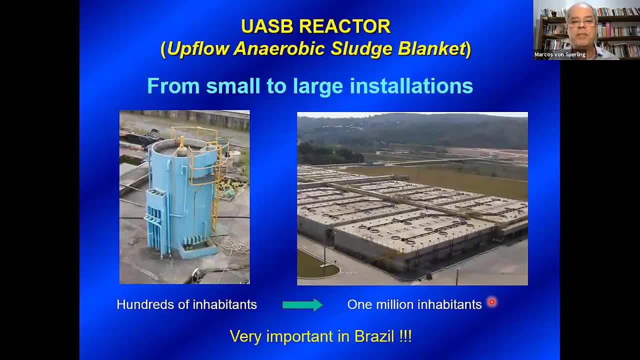 process. they take up a lot of area in this case here, for instance, three to six square meters per reactors and post treatment usb reactors. as we covered, they are widely applied in brazil. in some other countries they have some units in colombia, mexico also explore this. india they implemented. 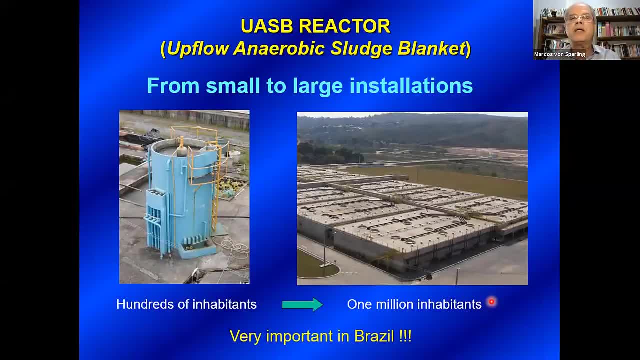 many and in all these countries there has always been a controversy: are they good, are they performing well? we can discuss this later on, but here in brazil they are used for small populations. this again in is in our research center. this is for 250 population equivalents. up to that's the, as far as we know, the largest uh treatment plant using usb reactors in the. 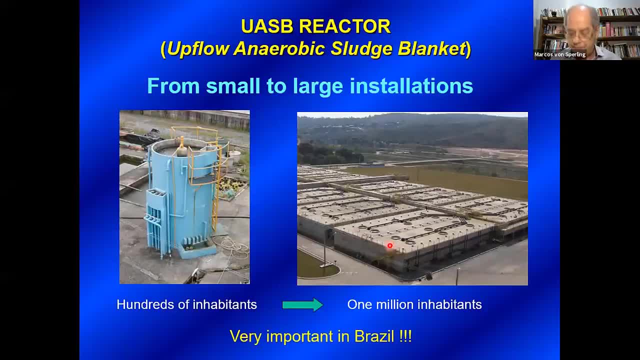 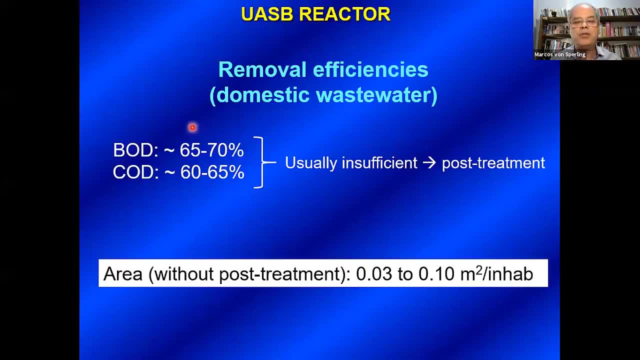 world for one million inhabitants. it's in my city here: bello horizonte, bello horizonte. okay, the removal efficiencies of just the usb reactors. they are not very high. that's a characteristic. this is not a disadvantage, this is a characteristic of the usb reactor. you can see. 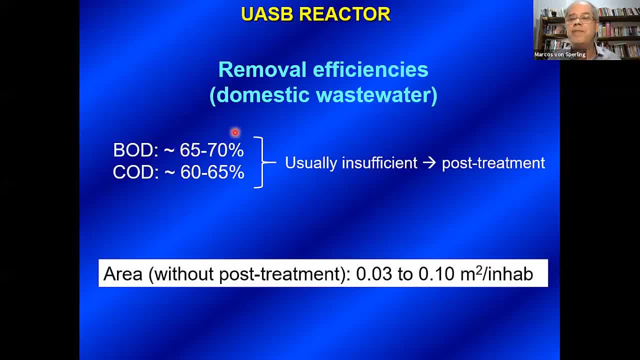 here that they remove between 65 to 70 percent of the bod, for instance, and now we have to think, okay, but they help a lot. now i have to think in terms of a post treatment stage. they are very compact. you can see here we started with uh, extensive systems, natural treatment systems. now 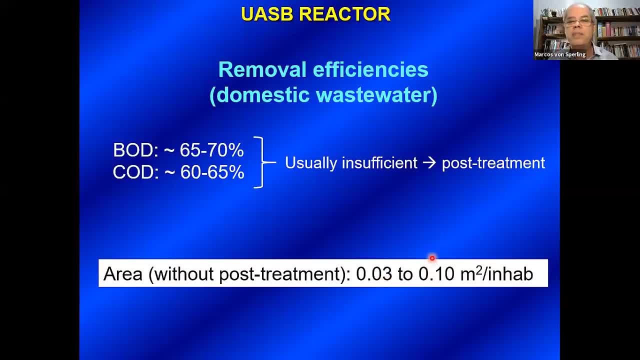 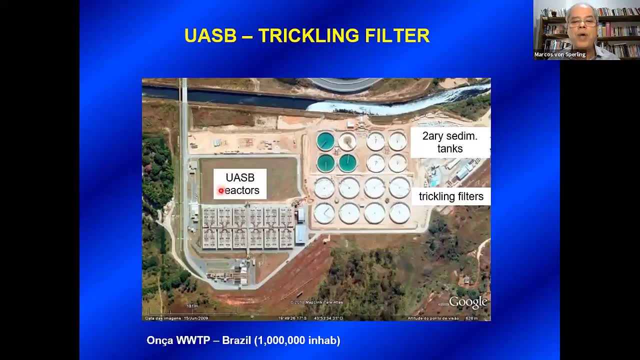 coming to a compact treatment system. the land requirements are very, very small. here in my city, bella horizonte, uh, as i told you, we have this large, this number of uh usb reactors comprising one million inhabitants, and the post treatment is by trickling filters. trickling filters is being 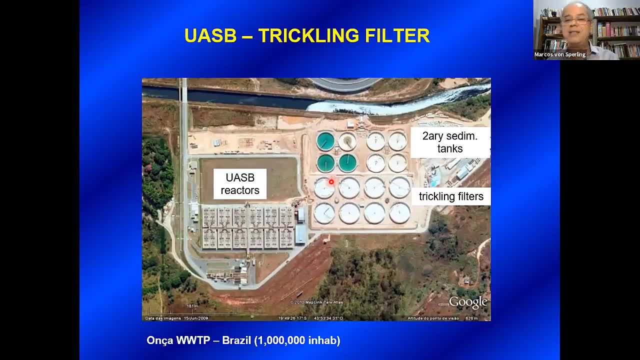 widely adopted here in brazil, in my state, uh, as well. uh, this is how i should say that it's- the automatic field treatment. precharging system is really one of the main features that people like to see. one may not already have access to it. some of them are starting normally here. they. 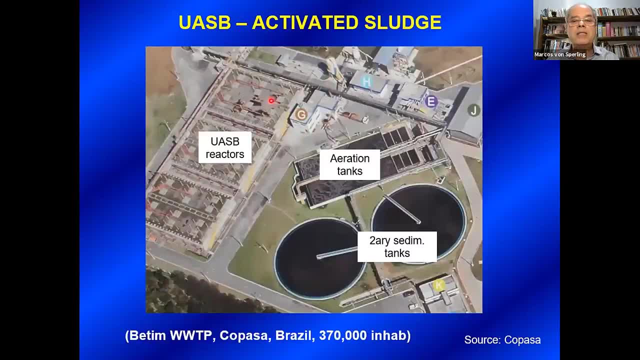 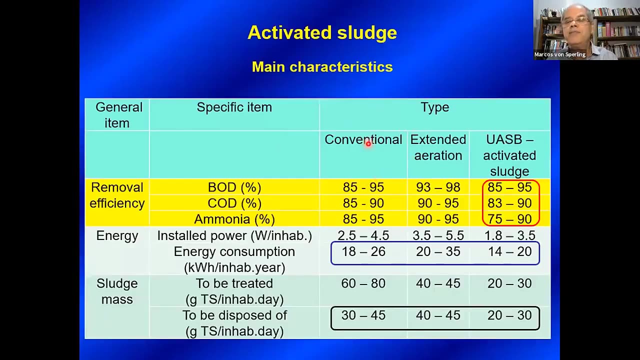 might no longer have access to this. four scolding to usb inhibitor: uh, the sepya pode the sludge. different alternatives, but we always have to remember about energy consumption. okay, The removal efficiencies are high, but we have energy consumption, But anyway. 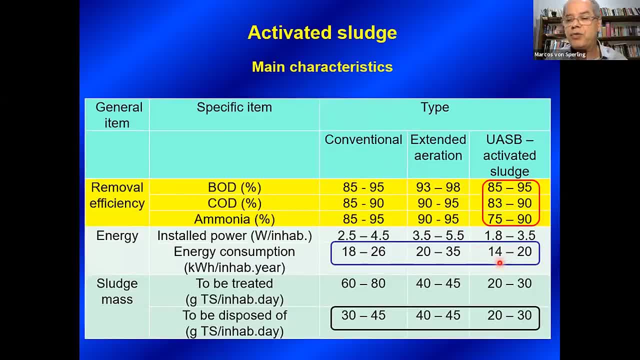 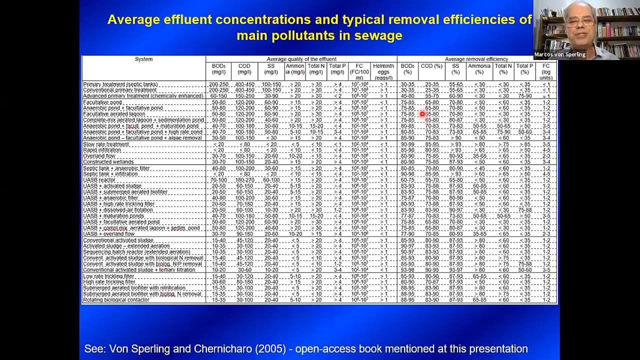 the arrangement of UASB reactor followed by activated sludge. among the possible arrangements involving activated sludge is the one which uses less energy and the one which produces less sludge to be treated and disposed of. Of course, we will not discuss about these tables here. This is just. 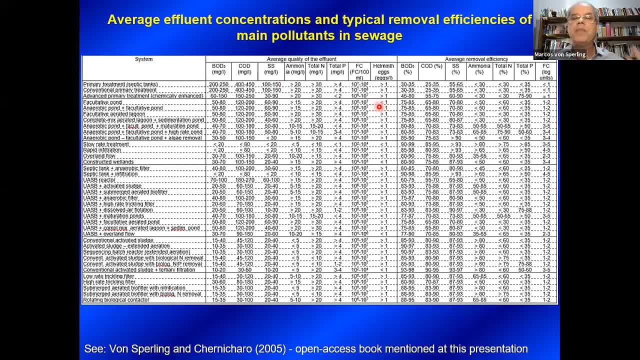 to show you that in that open access literature I mentioned to you, we have these summary tables for you to compare: many characteristics of many, many combinations of treatment processes: expected average quality ranges of values in terms of concentrations, in terms of removal efficiency. 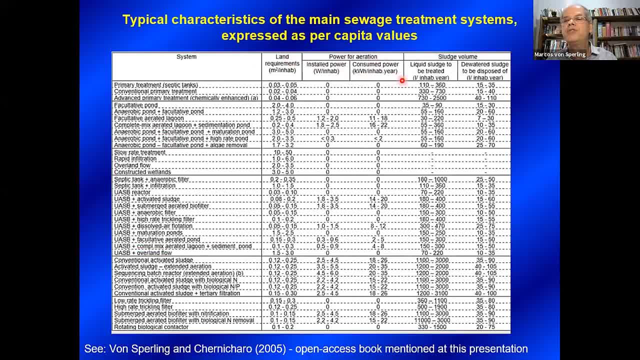 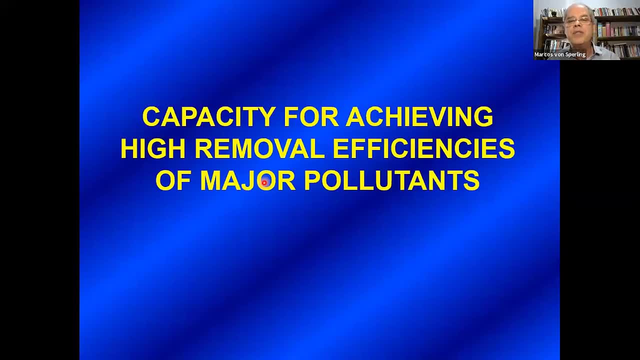 Land requirements, power requirements for aeration, sludge production and so on. So I think these are good summary tables if we need to make a very short comparison, a very quick comparison. Okay, Now, quickly, I will move and discuss with you about the capacity that these 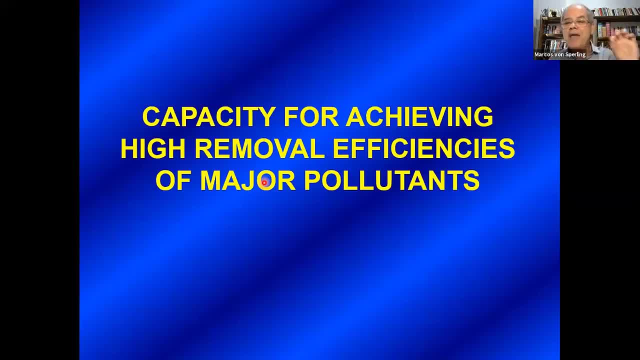 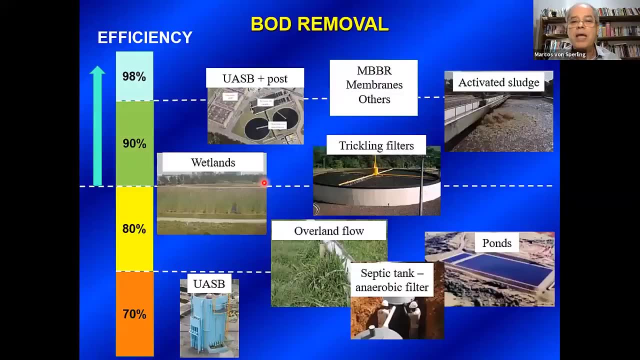 treatment processes have for achieving high removal efficiencies. So if we need to remove the major pollutants with a high efficiency, Okay, Let's start with organic matter. Express it here, for instance, in terms of BOD. So we start with low removal efficiency, moving up to 70%, 80%, 90% and coming up to 98% or even more. 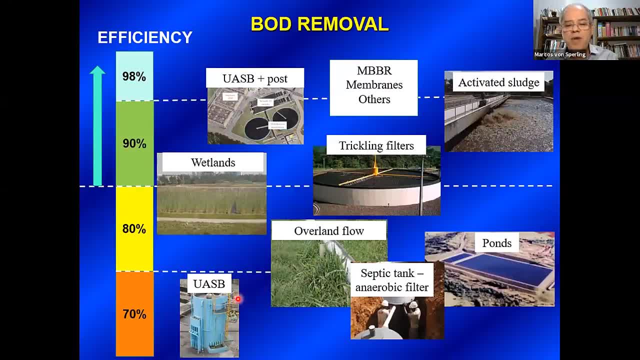 We have many possibilities, Some of them we have discussed here. So USB reactor stays in this range here. Septic tank followed by an aerobic filter in between. I have not discussed with you in terms of overland flow. It's another possibility- an extensive treatment process. 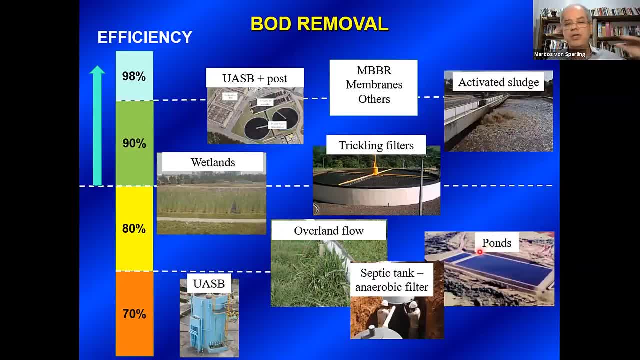 Ponds are not especially efficient in terms of organic matter, Wetlands more efficient, And then the compact systems: USB, followed by compact systems for post-treatment: trickling filters, activated sludge and, of course, more advanced treatment processes like moving bed bioreactors, those involving membranes, membrane bioreactors. 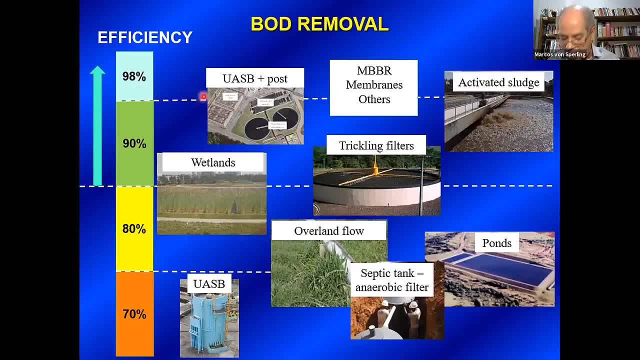 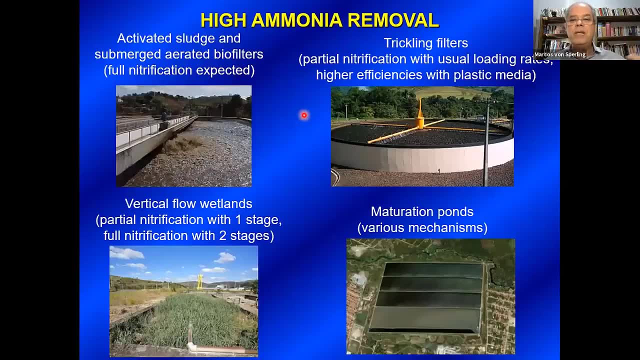 We will not discuss about them. Then you can reach high removal efficiency. If we need to remove ammonia nitrogen, the range of possibilities Decrease. Okay, Activated sludge, but it's not a simple treatment process. But you can achieve full nitrification. 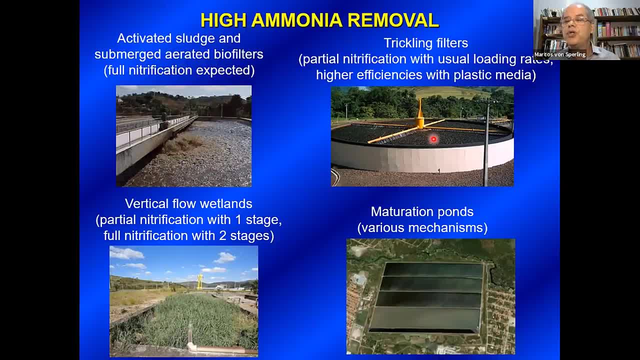 I rated biofilters as well, Trickling filters, which we have been advocating. they are very important. If you apply stones, crushed stones or gravel as support medium, you will not achieve high nitrification efficiency. But if you use plastic media and oxygen, 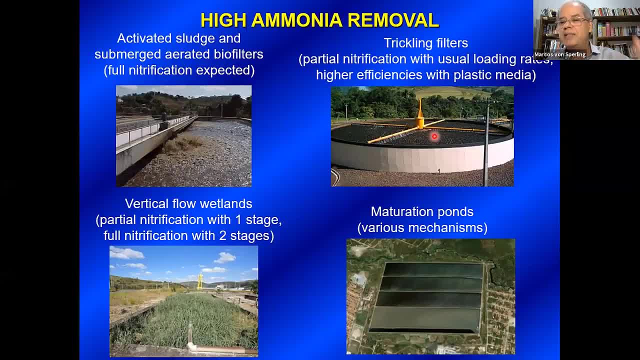 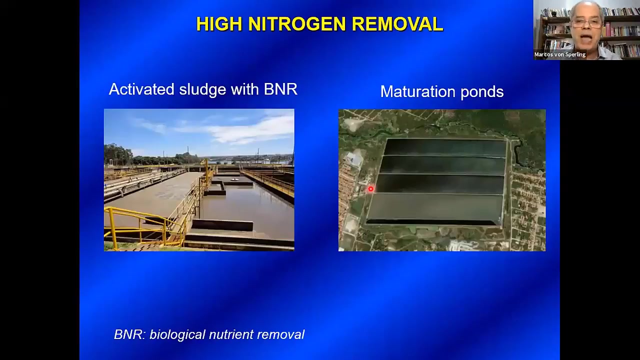 Also even better than plastic media, some sponge-based media. you can have higher nitrification, higher removal efficiency, Simple treatment processes like vertical flow wetlands or even maturation ponds. they are able to remove ammonia nitrogen. If we need to remove not only ammonia nitrogen but total nitrogen, so all forms of nitrogen, the range of possibilities decreases sharply. 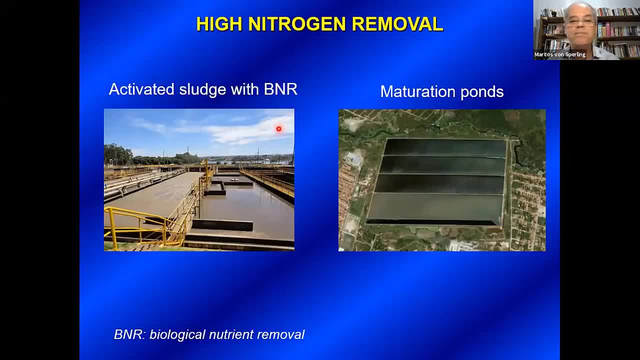 We could apply activated sludge with biological nutrient removal complex system, but also maturation ponds. They have been shown that they are good not only for removing pathogenic organisms, but they also remove nitrogen in the form of ammonia and nitrogen's total nitrogen. 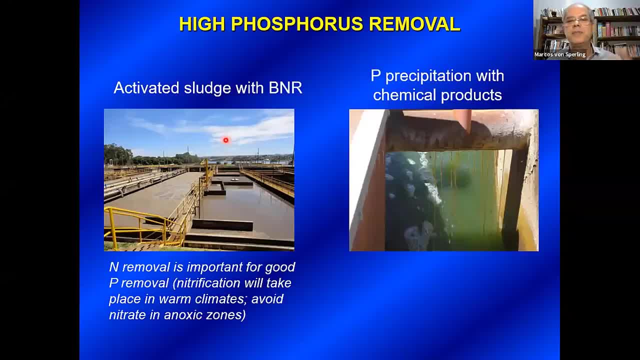 If we need to remove phosphorus, okay, activated sludge incorporating biological nutrient removal complex system. Reomb verbs also have a component. that have benefits. They can also remove pathogens from a soil. If you arrive an active�osporus, you can drive by. typically we don't have any foreign substances in native plants. 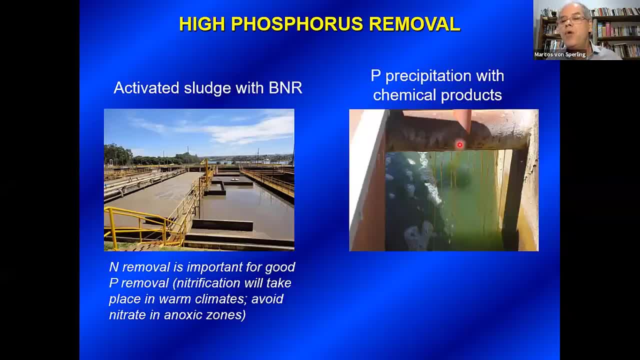 Just absorb things evil. One tendency and the only pathway if we would be affected is the use of anything. taymahirs 이렇게 administerwon detrimental substances in our produce- nutrient removal, But fortunately we have a chemical possibility If you add a chemical salt. 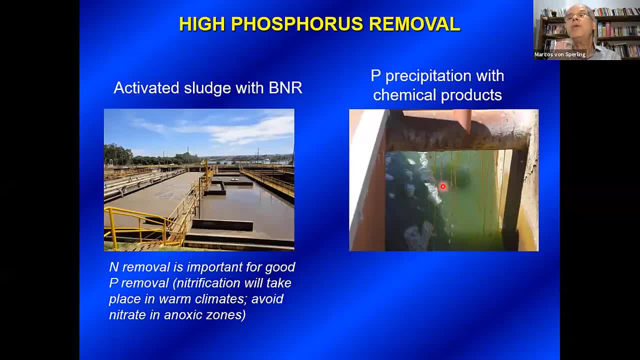 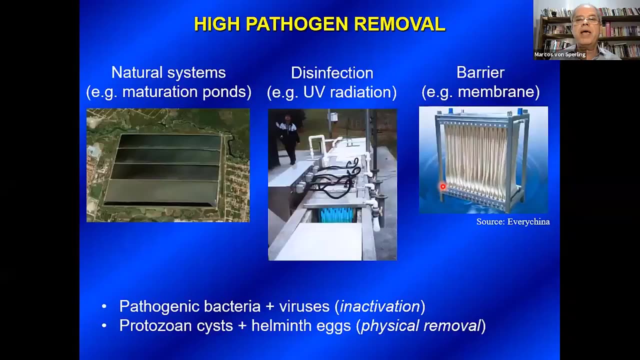 that precipitates the dissolved phosphorus, okay, we can solve the problem related to, for instance, eutrophication if we needed to remove phosphorus and if phosphorus was the major constituent causing algal blooms, Okay. and then, finally, in terms of disinfection, removal of pathogenic 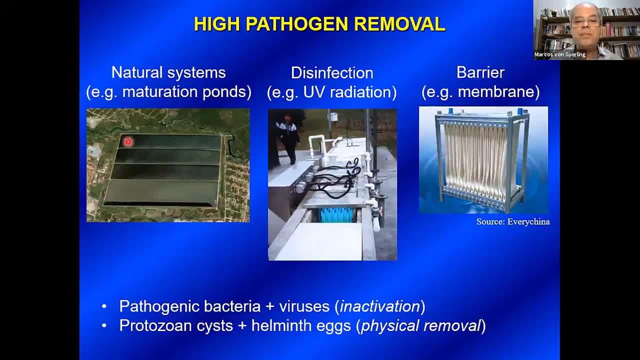 organisms. I emphasize again that maturation plants are able to remove the four categories of pathogenic organisms: pathogenic bacteria plus viruses via inactivation, protozoan cysts and helminth eggs. It's a physical removal by sedimentation, But of course you can apply. 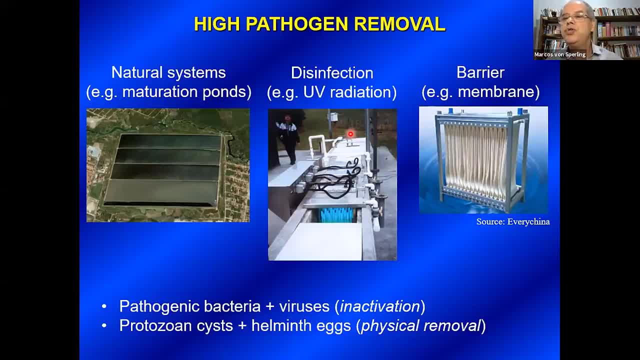 disinfection compounds to remove the pathogenic organisms. but of course you can apply disinfection compounds to remove the pathogenic organisms, But of course you can apply disinfection. for instance, UV radiation and membranes are fantastic because they are a 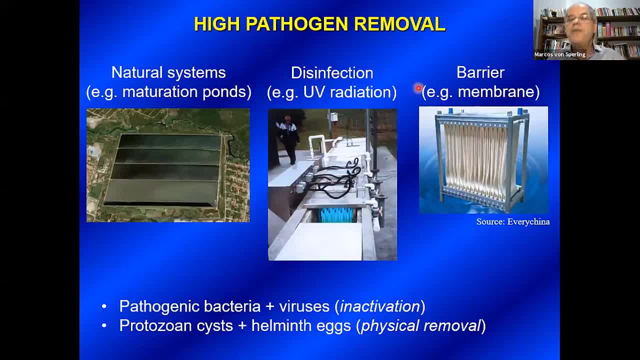 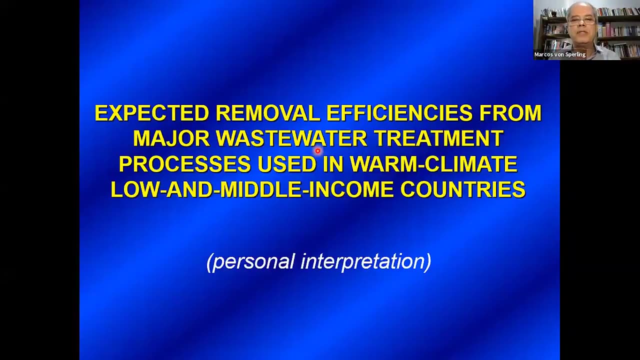 physical barrier. Now we have to think if we want to apply this in a low-income region. do we have good conditions for this? So that's the question I'm putting to you. And then, coming towards the end of my presentation, the last grouping of slides. 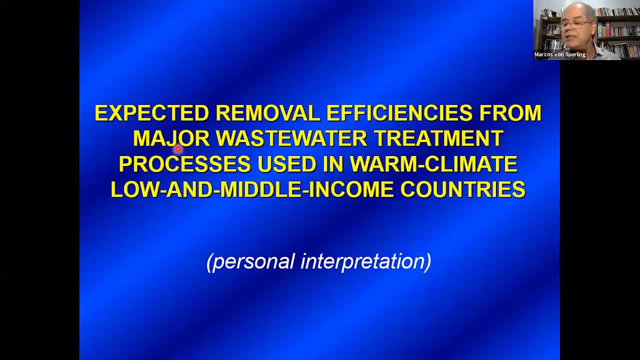 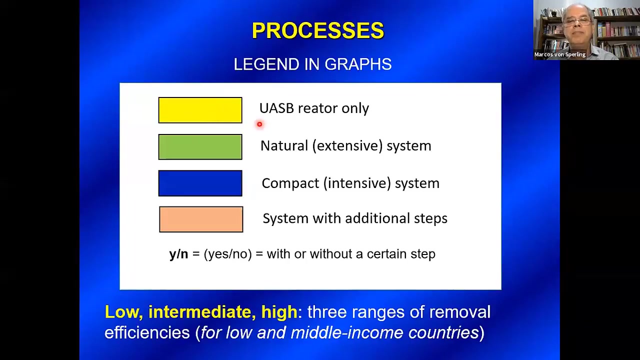 it's a personal interpretation of the expected removal efficiencies and I'm going to give you a few examples From the major wastewater treatment processes used in warm climate regions and low- and middle-income countries. okay, we will use this color scheme here: Yellow if we have only UASB reactor. Green if we are applying a natural 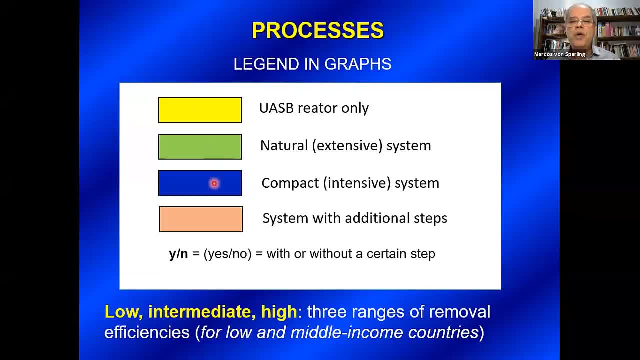 or extensive treatment system. Blue if it is a compact intensive treatment system. And then we are applying an intensive system as we described. And this other color, this pinkish color here is, if you add an additional step, like a chemical addition for phosphorus precipitation. 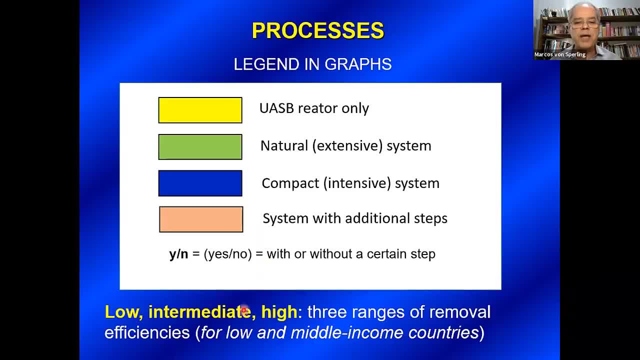 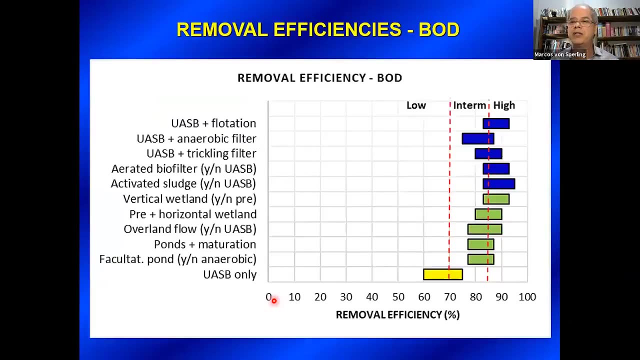 If you add chlorine for disinfection, okay, And I will show you in terms of low intermediate and high removal efficiencies. Thinking in terms of what is a high removal efficiency, I'm thinking about the reality of low- and middle-income countries. 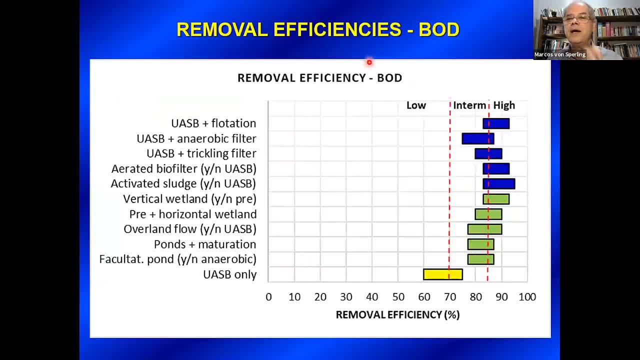 So it's a series of slides like that, covering the major pollutants, DOD removal, starting with the typical removal efficiencies. I will not discuss now, because I need to go fast now, about each individual possibility here. I would like to discuss about the grouping of alternatives. 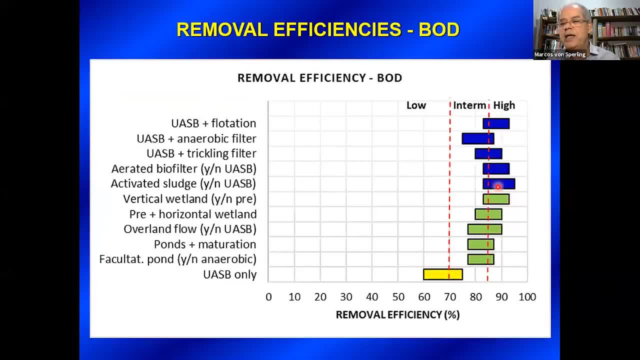 Yellow UASB reactor, In green the natural treatment systems And here the compact systems. It's a personal interpretation. I classified as high removal efficiency DOD removal efficiency which is higher than 85%. Okay, For high-income countries you could think, no, this is too little for me. 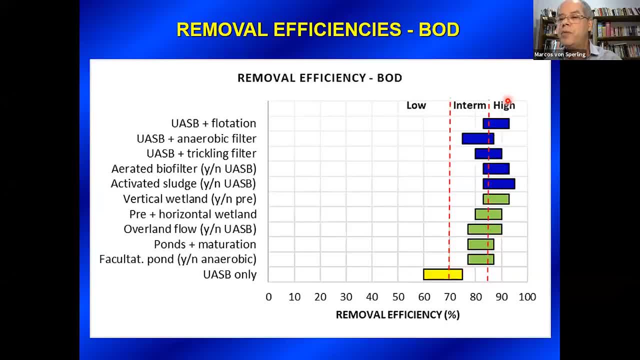 I would like to have 90, 95% DOD removal efficiency, But I think 85% removal efficiency for the reality of the countries I'm covering here is okay. Intermediate removal: I would like to have 90% removal efficiency, between 70% and 85% and less than 70% we could say low removal efficiency. 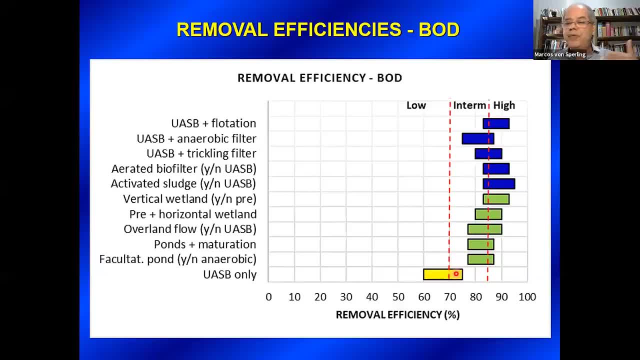 Okay, UASB reactor is in the boundary here, so UASB reactor alone cannot do a good job. And here you can see that natural treatment systems are able to provide removal efficiencies which are in some cases comparable to the compact systems. 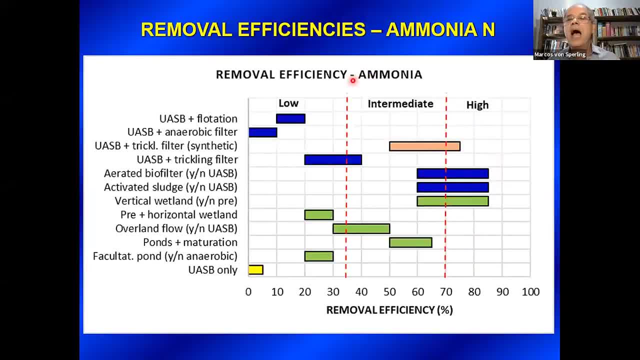 Okay, So that's important, But we need to think about the characteristics, Ammonia removal. Now, ammonia removal is more difficult than organic matter removal, So I classified here high removal efficiencies those which are larger than 70%, in between 35% and 70% intermediate. 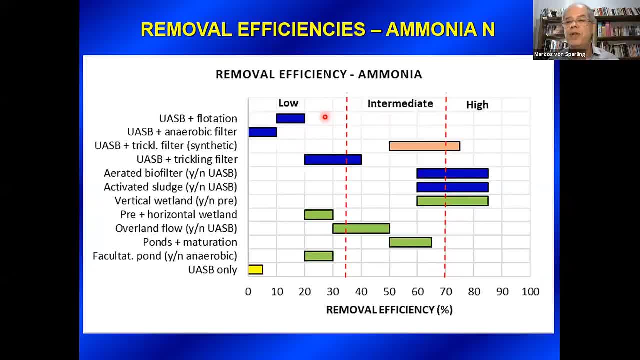 And lower than 35% low removal efficiencies. You can see here that, okay, now we have things scattered. Many treatment processes are only able to achieve low ammonia removal efficiencies, regardless whether they are compact systems or natural treatment systems. Others achieve intermediate removal efficiencies. 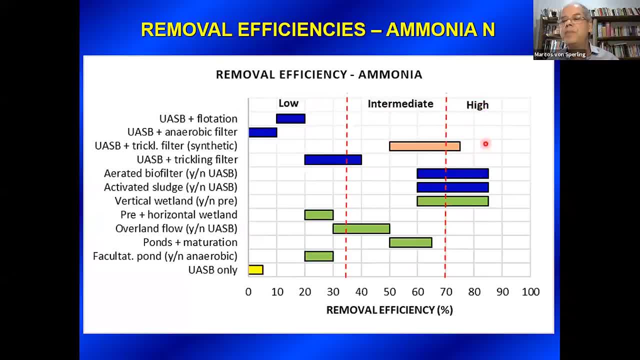 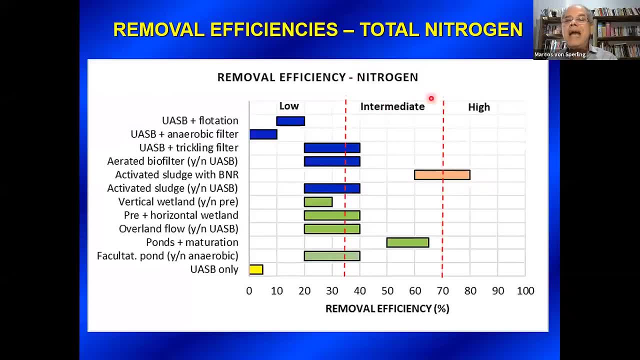 and only a few of the treatment process are able to achieve high removal efficiencies. We have natural systems and we have compact systems. Nitrogen removal- total nitrogen removal- is even more difficult And most of the treatment processes are able to achieve only low removal efficiency. 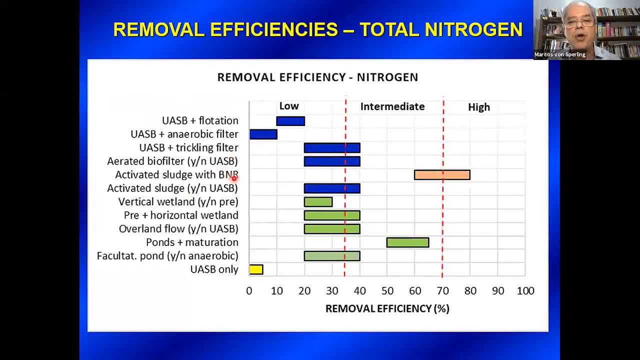 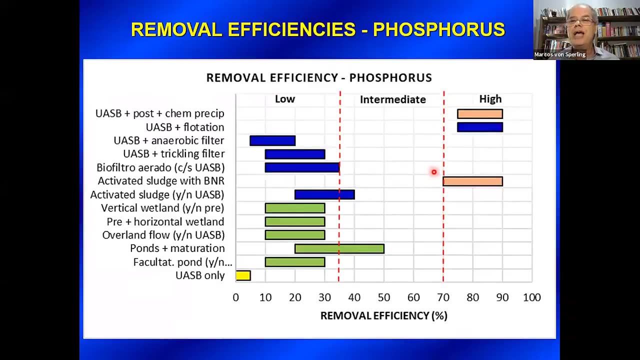 unless you implement something like biological nutrient removal okay, And then even intermediate removal efficiencies only say ponds, followed by maturation ponds. So that's a problem. We have to think about this when we establish discharge standards. in our country, Phosphorus. 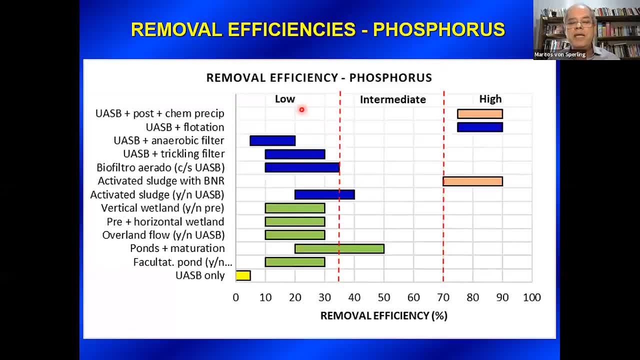 the discussion is somewhat similar. Biological means very few treatment processes give us high removal efficiency. Most of them will give low removal efficiencies, but fortunately we're able to get to use processes that give us removal efficiencies If we add chemical precipitation followed by flotation and so on. 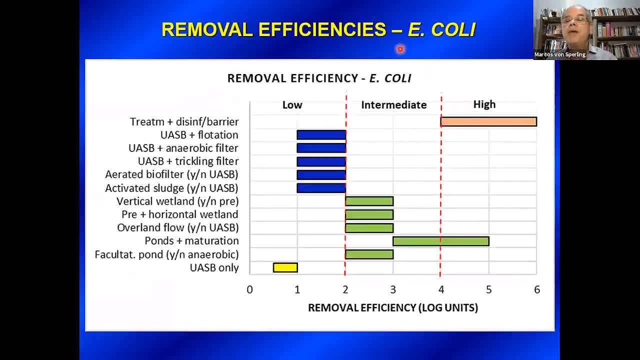 and biological nutrient removal. okay, Pathogenic organisms. I will not cover all pathogenic organs, just the main indicator organisms, Escherichia coli, representing pathogenic bacteria, Most of the compact treatment process. they do not have important mechanisms for pathogenic bacteria removal or for virus removal. 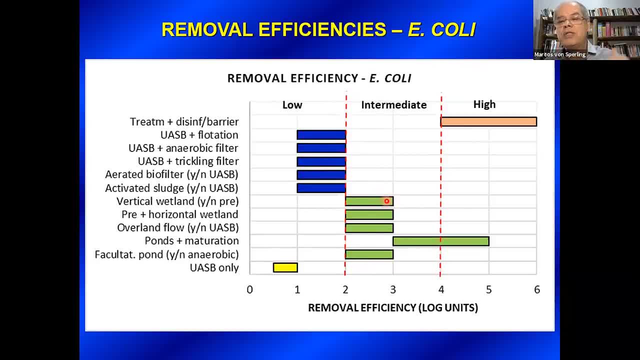 The natural treatment processes are more efficient because they have longer retention times. They have longer retention times And more mechanisms. And, of course, as I told you, if we incorporate maturation ponds, we are able to achieve high removal efficiencies. And, of course, if you include, 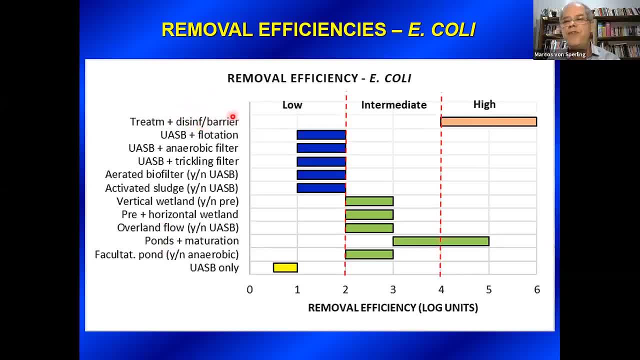 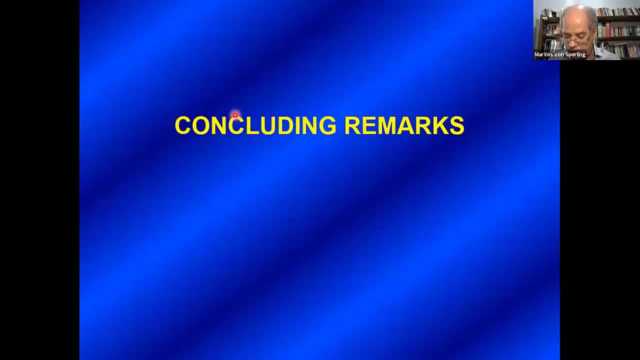 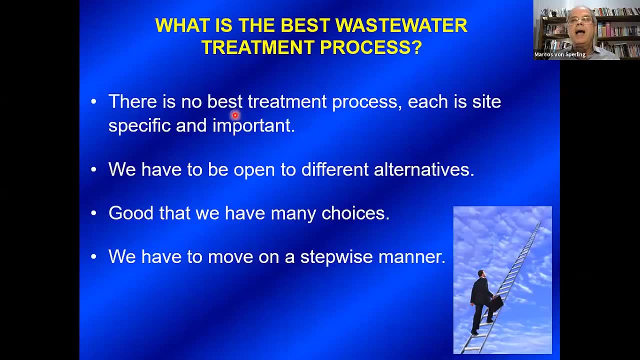 in any of these treatment process, one stage for disinfection, or a barrier like membrane. okay, you can do a good job. So my concluding remarks would be: what is the best treatment process? Because after presenting so many possibilities, it's natural that we think what's the best. 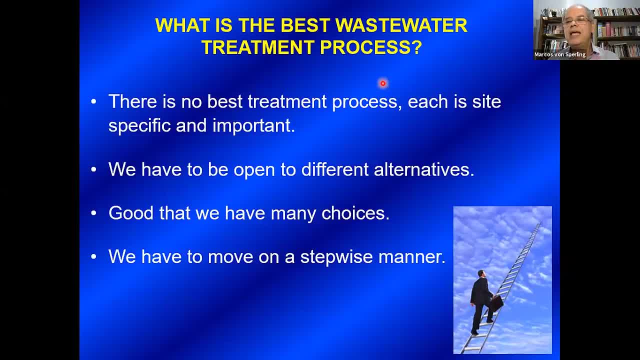 There is no best treatment process. Each is site specific and each is very important. So we need to do very good studies, conceptual studies, to select in each case what is the best treatment process. We have to be open to different approaches, Different alternatives. 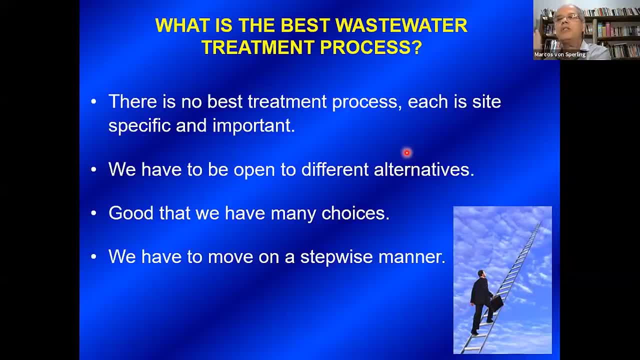 I cannot say: well, I will use only this treatment process because I like it, Because under other circumstances you will need to apply a different alternative. It is very good that we have many, many choices. If you remember that large table I showed you. 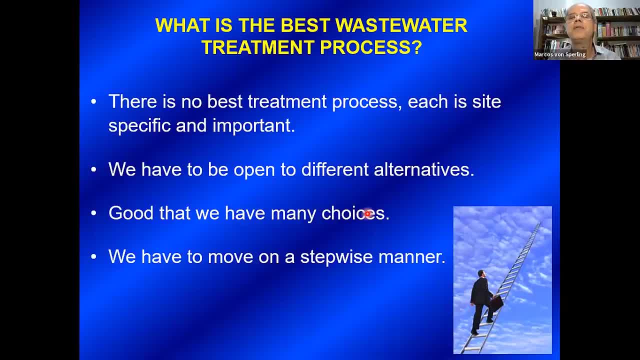 they showed more than 20 combinations of possibilities that can be applied under our circumstances: Either simple treatment, more complex treatment process or more complex treatment process- But we do have the choices. Okay, So many challenges. we started discussing about challenges. How can we solve this?